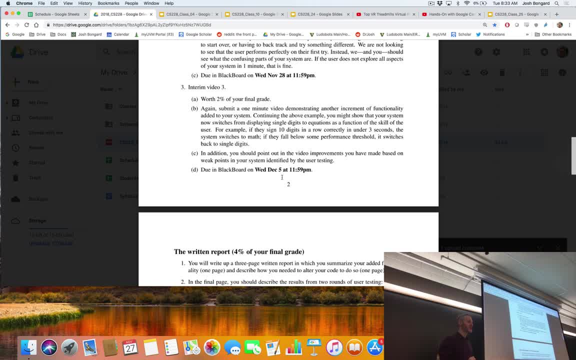 If we had more time, we'd have you do another round of user testing, but what we're looking for in the interim videos is that obviously you're putting in some of your own creative ideas about how to make your system more usable for a wider range of users. 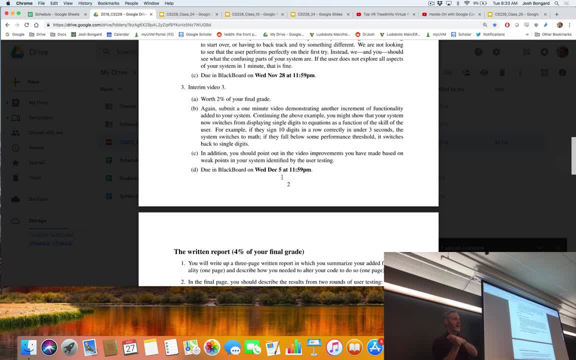 and that you'd like to see that You learn something from user testing and that is feeding back into your system. You'll remember back towards the beginning of the semester when we talked about the process of design for HCI. We had sort of this star pattern and at the center of the star pattern was user testing. 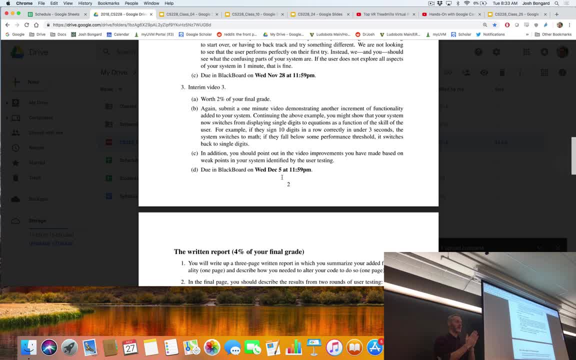 If you go and work in a production house on any software that's going to be exposed to the users, if you do any aspect of the front end of a large-scale system, you do a lot of user testing. And one of the interesting things about user testing is often what you thought was intuitive turns out to be non-intuitive, and vice versa. 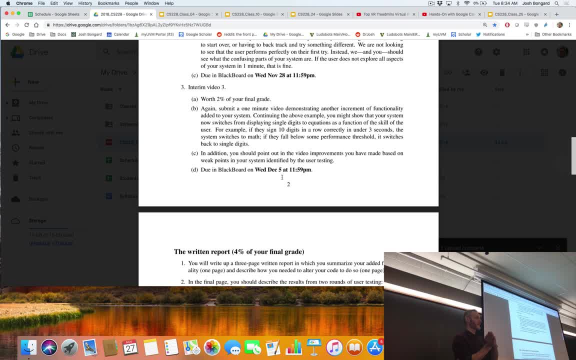 Did anybody have that experience with their users? More or less Okay. So it's also a learning experience, not just, obviously, for your users, but for you. So we're looking again in interim video two, not that your users had a perfectly smooth interaction with your system on the first try, but that you are capturing these moments in which they're confused, frustrated. 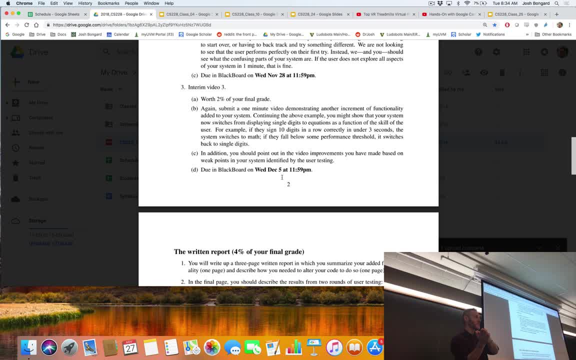 or surprisingly at ease with this particular aspect of your system and then addressing that in interim video three. All good. Any questions about the interim videos? final project: So far, so good. Yes, So when you say sign 10 digits in a row, frankly does that mean you're going to display 10 different numbers in a row? 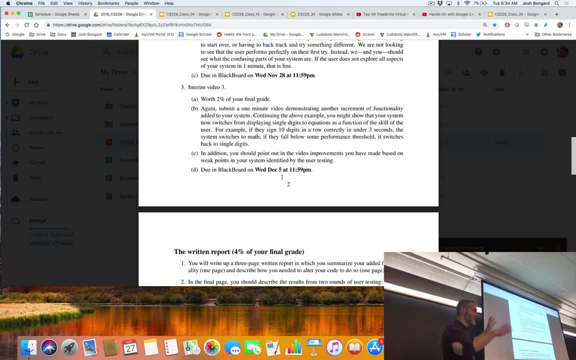 This is an example, right? So this is just following this example of, in this case, this hypothetical, This hypothetical, So a student decides to show sequences of digits and then the users have to sign it: Or 6,, 7,, 4,, 3,, 1,, 2.. 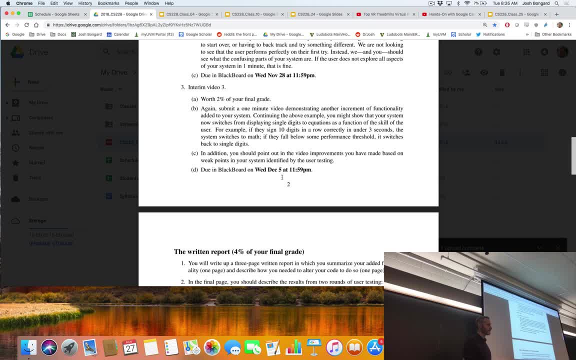 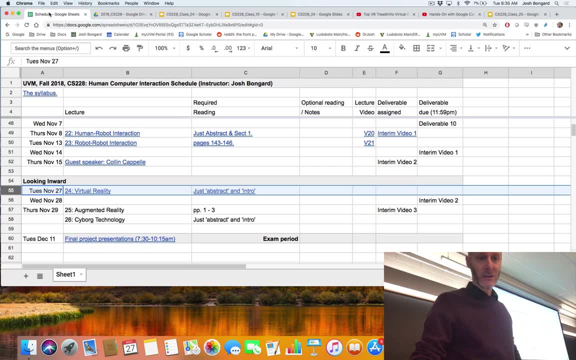 Again, that's just an example. That may not be what you're actually doing, Any other questions? Okay, So back to lecture. And again, it's been a week, so let's reorient as to where we are and where we're going. 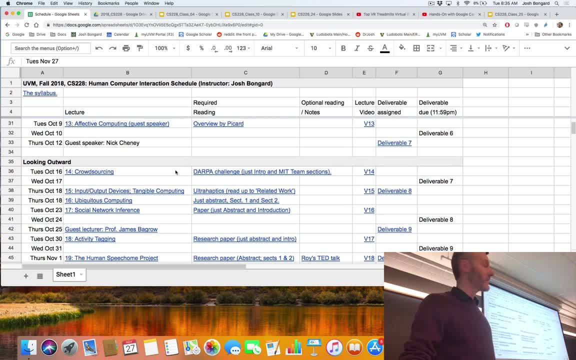 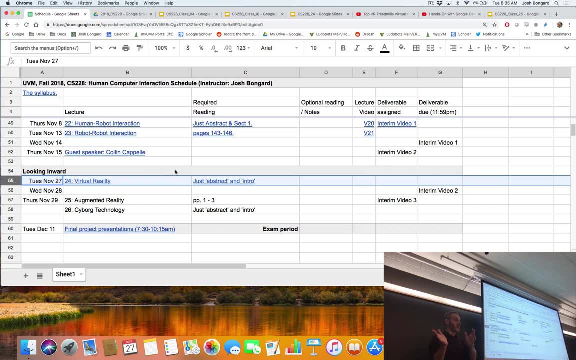 We concluded, before the Thanksgiving break, this long section on looking outward. This is a great time to be studying HCI and for those of you that go and work in a software production house, it's a great time to be working and actually developing HCI, because our society is in the process of stitching technology into the real world, right. 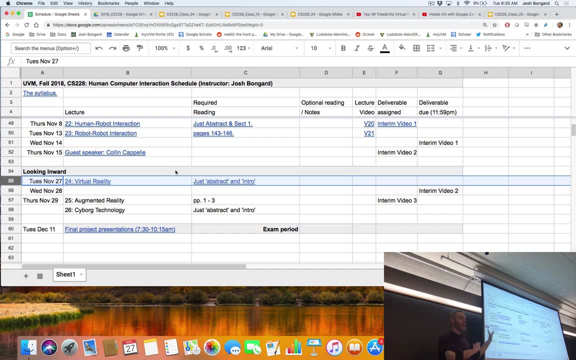 Ten years ago and 20, 30 years ago, we figured out how to build these things called computers. We figured out the Internet. Now we're figuring out how to expose all of these devices directly to the real world. So we talked about embodiment. 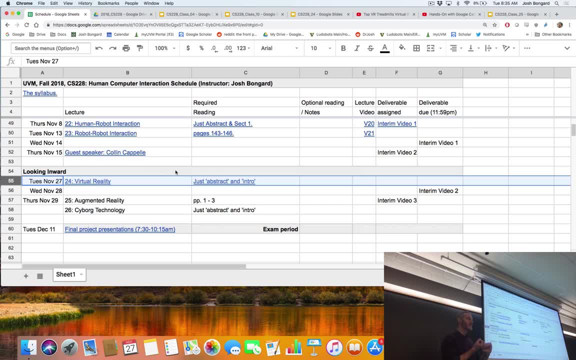 We talked about embodied cognition, situated cognition machines that are drawing data directly from the real world And, in the case of robots, are starting to be able to move about in the real world. And as they do move about in the real world, they have control over the kind of data that they receive right. 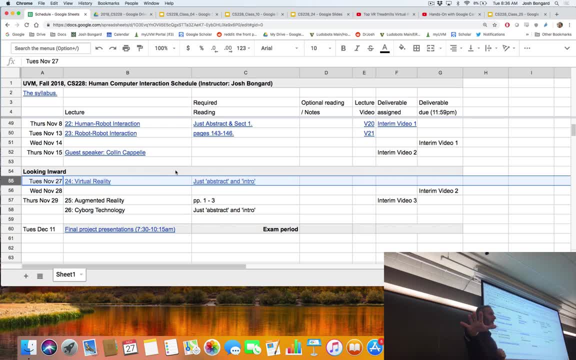 Very, very different from a laptop that sits passively on your desk and waits for you to type something or waits for a packet to arrive via the Internet. So We're in the process of instrumenting technology into the physical world. At the same time, we are getting better and better at creating virtual worlds and more and more of us are spending more and more time in those virtual worlds. 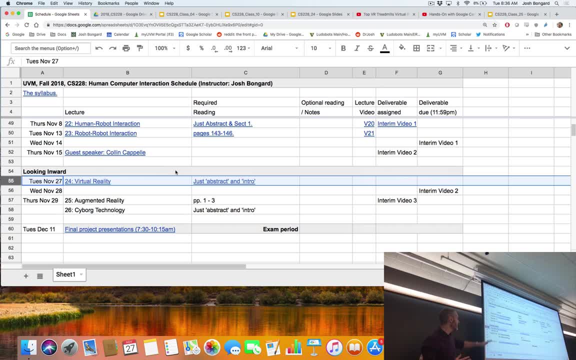 So that's what we're going to look at in Looking Inward. We're going to spend today talking about virtual reality, where we enter to some degree into a virtual world. We may finish lecture 24 today. We may start lecture 25 on augmented reality. 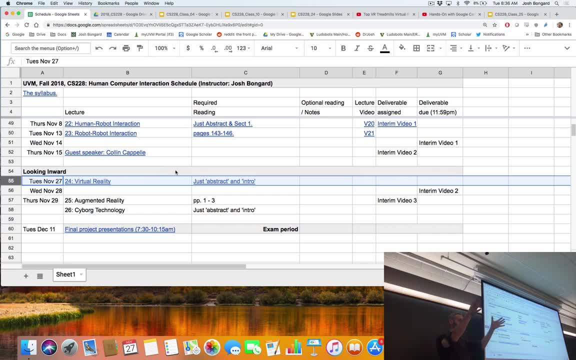 Where we have a human observer who is viewing and possibly moving about in the real world And as they do, we are layering virtual reality on top of physical reality to give us augmented reality. And in lecture 26, we'll look at a different form of inward facing technology. 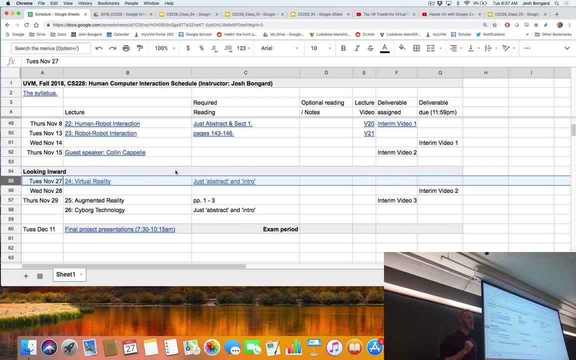 Inward, literally into or under the skin, into the human body. So what happens when we have a human nervous system, A nervous system talking directly to technology and possibly the technology speaking back directly to the nervous system and skipping over our five senses, right? 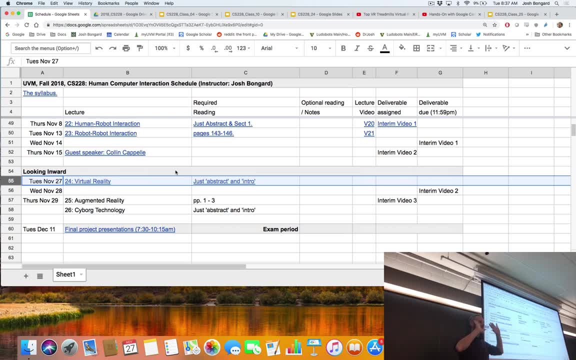 In virtual reality and augmented reality. whatever you're looking at, it is over or on the skin. Cyborg technology under the skin. That's the distinction we're going to look at today. Okay, So let's talk about Looking Inward. 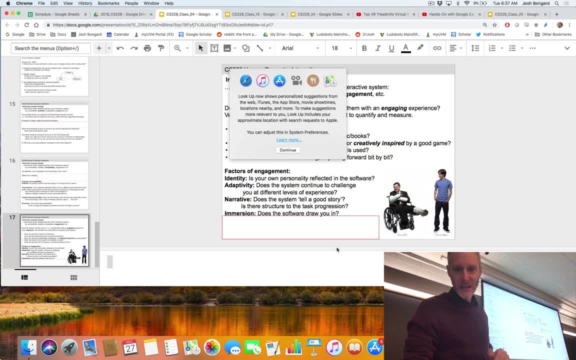 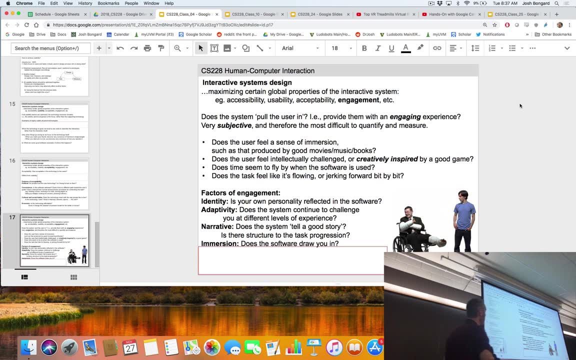 As we're going to Before we do, just to sort of set the context again. You remember back. you hopefully remember back towards the beginning of the semester We were looking at, when we were talking about interactive systems design. We were talking about trying to design software that is not just correct and bug-free but has these additional non-functional requirements. 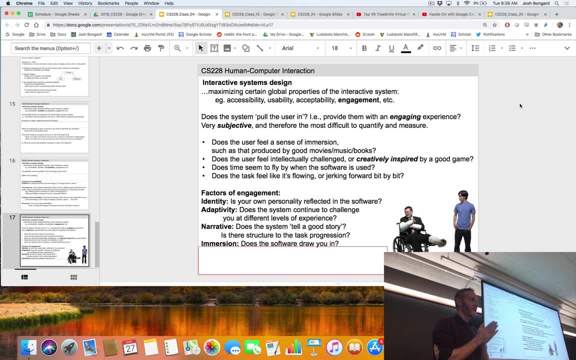 They're not related specifically to the function of the software itself, but these more general and somewhat vague properties Like the system should be accessible, usable, acceptable. And the last one we looked at is the most subjective of them, which is engaging. 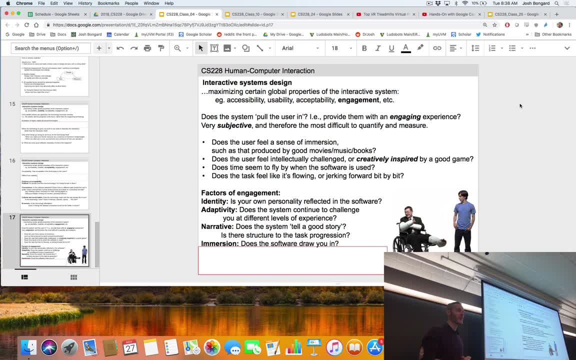 So if we're creating a computer game, for example, it should be not just bug-free and accessible to all and easy to figure out how to play the game, But it somehow draws the user in, They feel engaged or immersed inside that world, right? 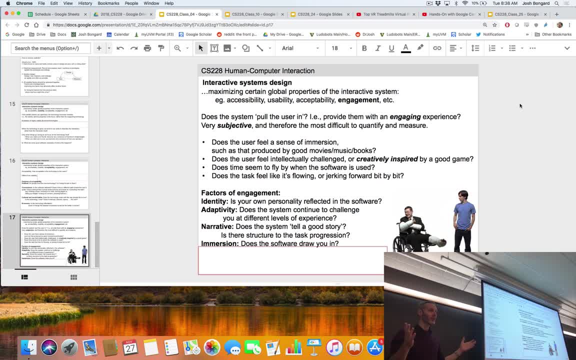 We've had virtual reality for a long time. It's called books, or theater, or music, or culture or art. Now we're figuring out how to do it with technology, But what art and virtual reality which we're going to look at today? what all those things have in common is they're able to pull someone into that virtual world. 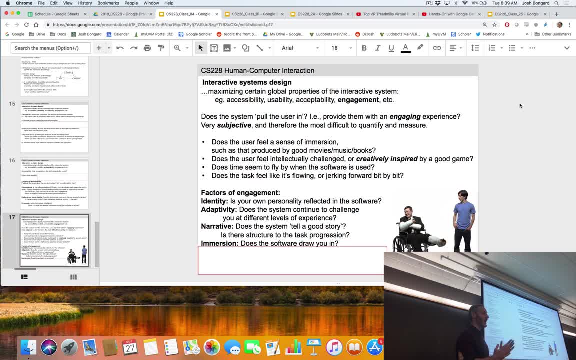 Art's been around for a long time. It's very popular. Computer games are becoming increasingly popular, So there is something about the human psyche that loves this process of being pulled into these virtual worlds. Right, We love a good story. We love a good movie. 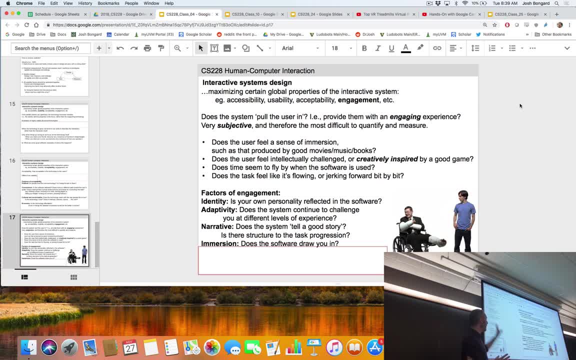 We love a great piece of music where we lose ourselves in it. So for the why of virtual reality, why do we go about building it And why is it so engaging to so many people? is we have this desire to be drawn into another world? 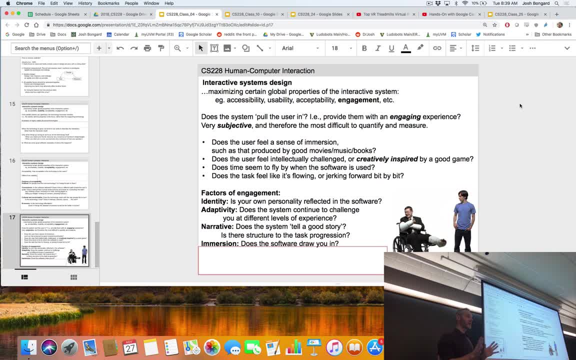 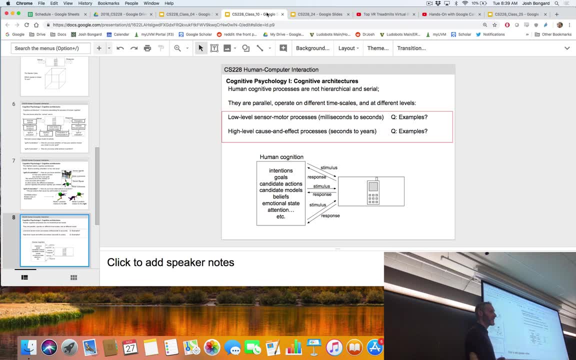 That's the why. If we do want to try and create virtual reality, then we can switch and start to think about the how. How do we create virtual reality? That's engaging You? remember back to I forget which lecture. this was our lecture in cognitive psychology on mental models. 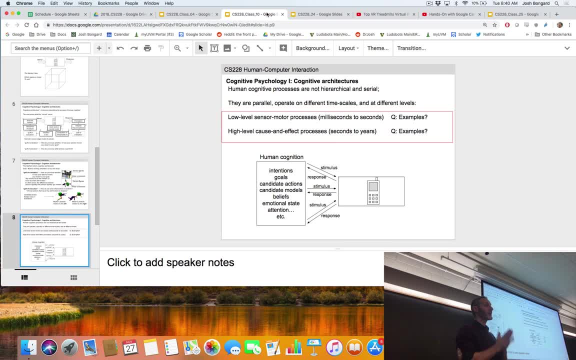 If we want to try and create an illusion. what distinguishes virtual reality from all the art that's gone before is that we're going to actually try and put the actor, the observer, as a participant, an active participant, in the virtual world. 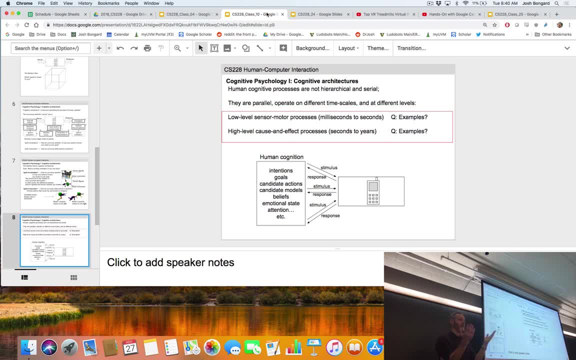 Typically, when you read a book or watch a movie, you're sitting quietly, you're sitting still, you're interacting with the story in a minimal way, You're moving your eyes and saccading across the page or across the movie screen, but otherwise you're passive. 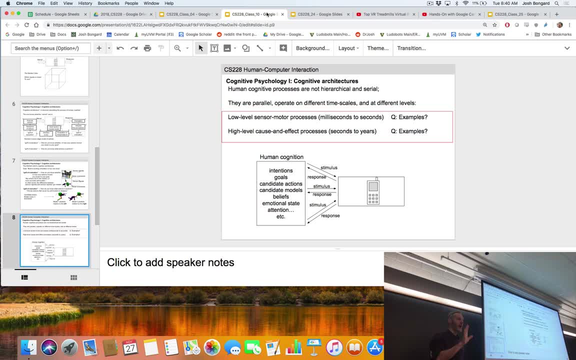 Virtual reality systems are trying to engage more and more of your sensory and motor systems. So how do we build a mental model of a story or a computer game? If we're going to be active, we are going to move. We move in some way and our mental model of the virtual world which we feel that we are experiencing, that mental model, predicts what the sensory repercussion to our action is going to be. 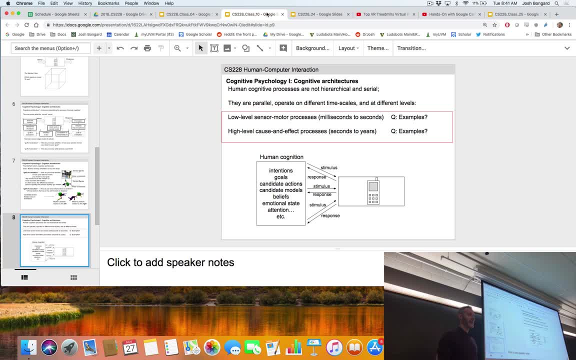 As far as I know, I'm in the physical world right now and if I take a step to my left, my mental model of the visual scene in front of me predicts that all of your heads will move one step to my right, Right. 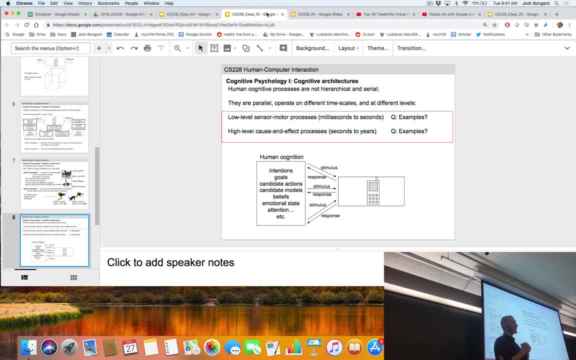 If I'm wearing virtual reality goggles and I take a step to my left, my mental model of the visual scene in front of me predicts that all of your heads will move one step to my right, Right, Right. If I take one step to the left. what I'm seeing on the inside of the goggles, what does my brain predict is going to happen to that visual scene? 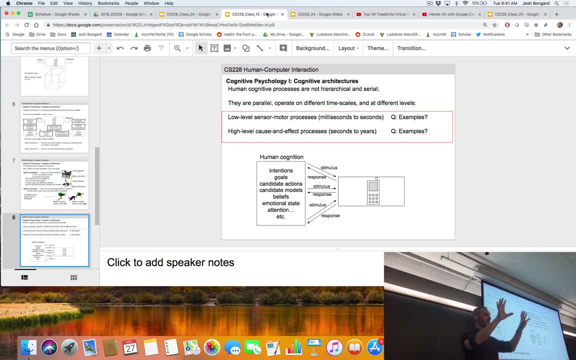 Same shift, Same shift, right. So the scene that is painted onto the monitor on the inside of the VR glasses is going to have to shift to the right. How do the glasses know to do that? How do they have a position to take? 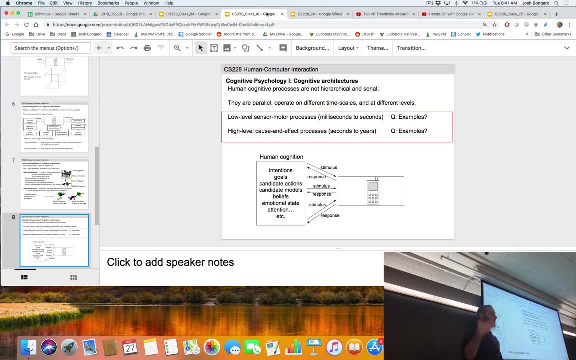 Position. They know that somehow the virtual reality system is going to have to sense my movement, Right? So we're back to a social robot, if you like, where the human moves, The output of the human becomes the input to the technology- in this case VR goggles- and then the VR goggles outputs something, changes the visual scene, or makes a sound, or vibrates, does something else. 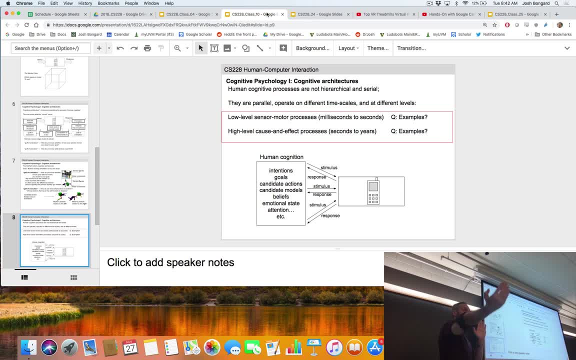 which, because it's being worn by the human, becomes the input to the human. around the VR goggles Correct, and around and around and around we go right. the interesting thing about virtual reality, of course, is there's lots of different ways that i can move and interact with the physical world. 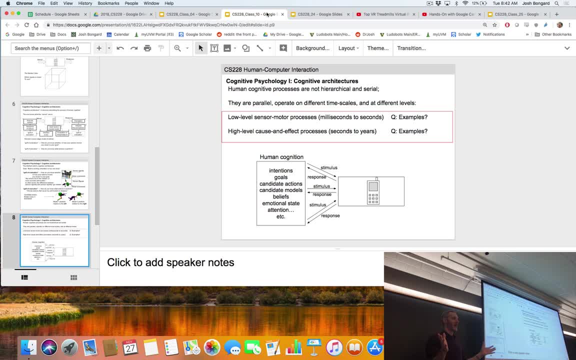 how many of those can be sensed and captured by a vr system, and for how many of those actions can the vr system give me back the sensory repercussion that i expect? tricky right, some are easier than others. if i'm wearing goggles and i move, that's relatively easy to capture, as long as there's an. 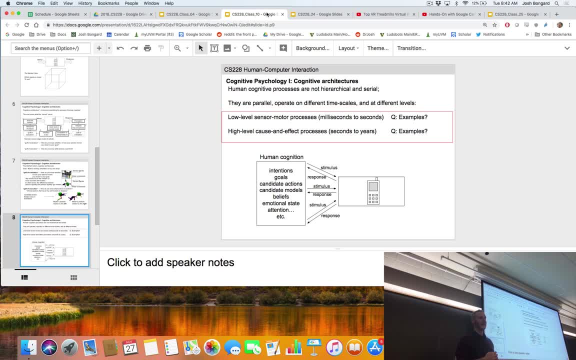 accelerometer or something that detects motion in the, in the goggles. that's going to be relatively easy to capture. what is much more difficult to capture: touch, absolutely right. so unless i'm wearing gloves- vr gloves- that's going to be a little tricky. what else? what's more tricky than? 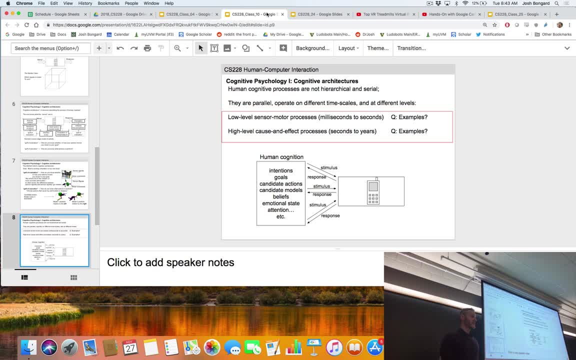 just head motion, smell, smell, that's. that's going to be tricky. yeah, walking- right, we're going to look at walking. i see a virtual world in the inside of my goggles and i want to walk through that environment. i start walking in the real world. how is the vr system going to to deal with that? yes, responsive sound, that's going to be. 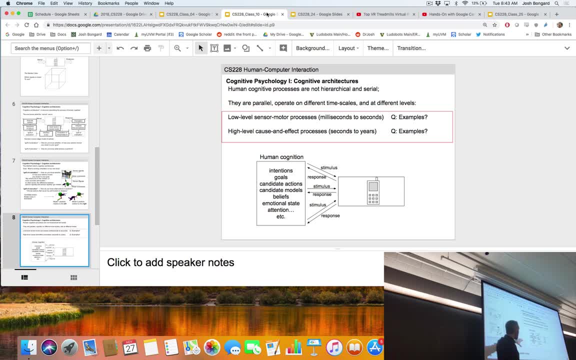 tricky as well, right? so when we're going to look at a number of vr systems today- and as we're going to look at a number of vr systems today, we're going to look at a number of vr systems, we do. I want you to keep this cartoon in your mind, your brain, or the person who's. 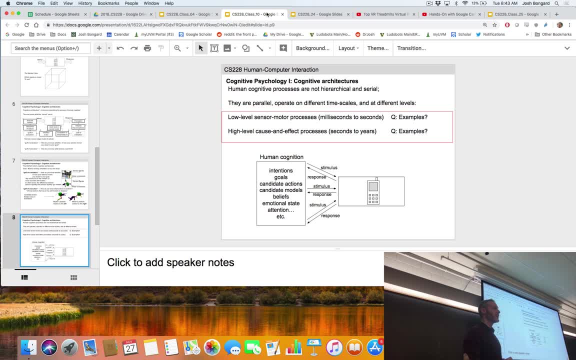 wearing the VR system. their mental model is going to be making lots of predictions for different sensory systems. as I move around, not only does the visual scene move, but I hear my boot falls in the background right. there's a lot of different things that are going on. some of them are a little bit of more. 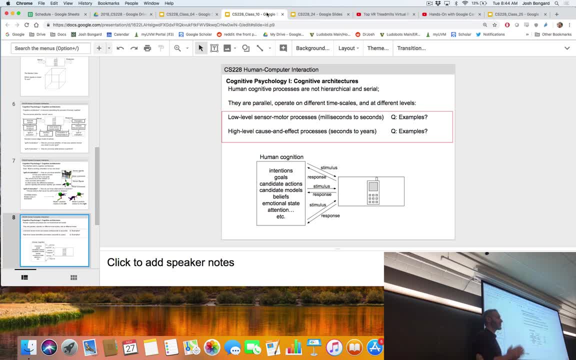 obvious than others. so our brains are making predictions about sensory repercussion for lots of different kinds of action: head movement, body movement, touch reaching, grasping and so on. smell another good one and then at the same time we're also making predictions about those repercussions. so repercussions across lots of different sensor modalities, or across our five. 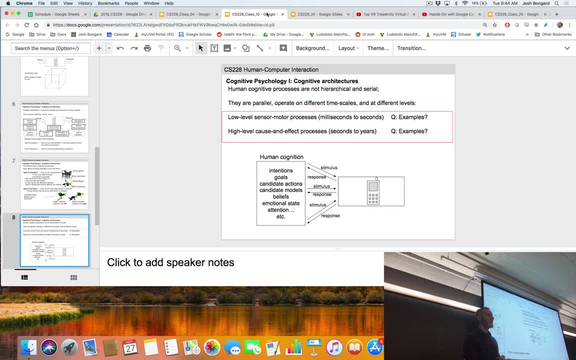 senses and, most importantly, our expectations have a timestamp associated with them. we have an expectation about how soon we're going to receive something. we're going to receive something. we're going to receive something. that response- one of the things that's made VR so tricky for so long is most of 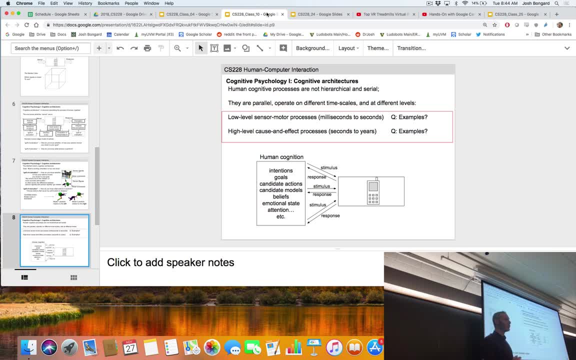 our predictions are in real-time. if I were to move, and to the left, and my visual scene move to the right a tenth of a second later, no good, right, it's happening in real time. from my point of view, there is absolutely no lag in my movement and the sensory response to that action. that's true for most of. 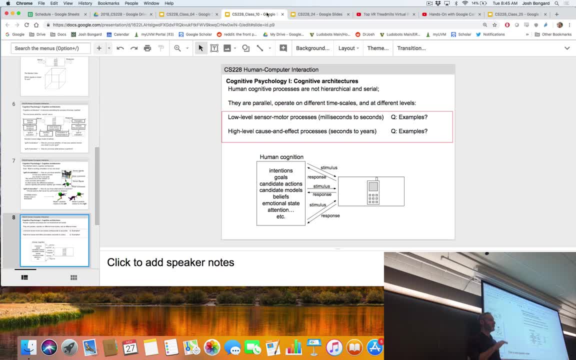 the actions i can perform in the physical world, but not true for all of them. where are there some actions where i actually expect a leg, an echo, an echo, absolutely? this room is actually a good example for that. there's a slight echo in this, this room. what else kind of related, but like sound? 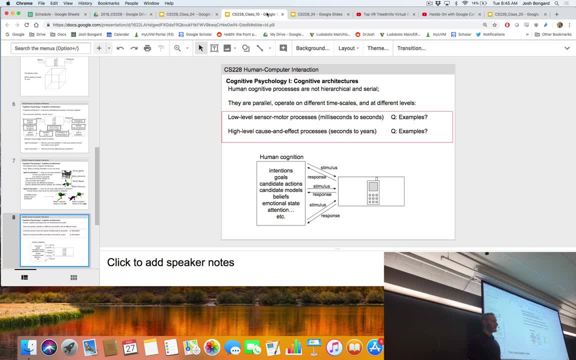 over distance to the purpose, absolutely right. so most vr systems, they're projecting a 3d scene onto your retinas, so we have an expectation about the three-dimensional world, absolutely okay. so tricky right. we're making- uh, we're making- predictions about lots of different kinds of 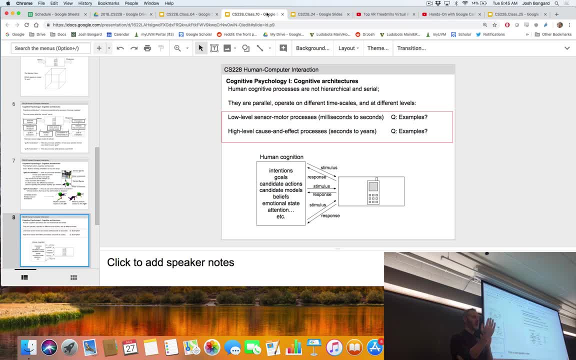 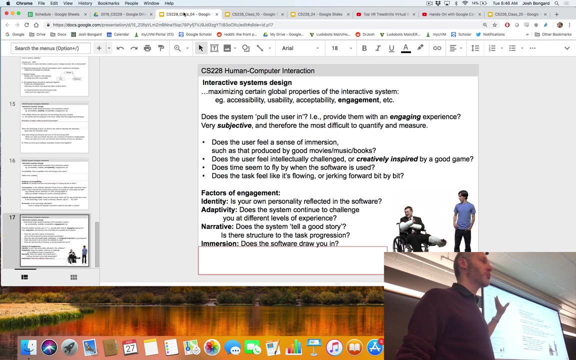 actions across different sensor modalities at different time, lags or, in a lot of cases, no lag at all. how much of those expectations can a vr system meet? okay, so that's the how of vr. very tricky, and we're doing it to try and match this. why we're trying to cast an illusion. we want to make a world in which 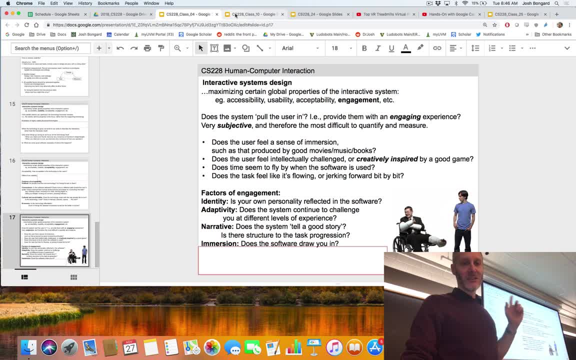 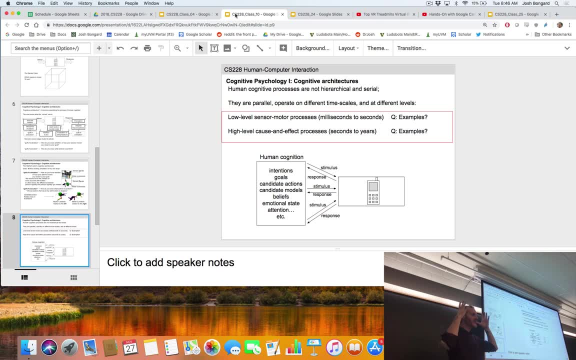 someone feels drawn into it and lost in it. in the videos we're going to watch today, you'll hear them talk about breaking the vr illusion. you feel that you're in the real world. you put on the glasses. the glasses haven't been turned on yet. you're still in the real world. you turn on the glasses. 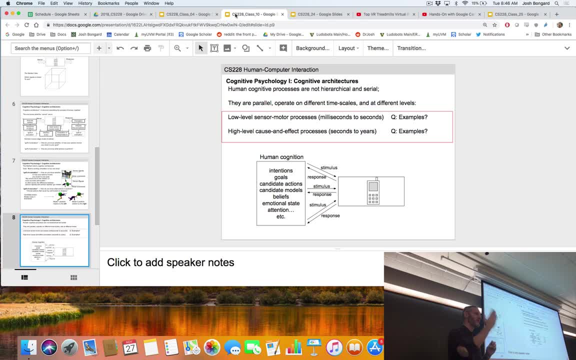 and if things are working, you turn on the glasses and you're still in the real world. at some point, you no longer feel that you're in the physical world, you're in the virtual world. right? what needs to happen on the VR side, on the technology side, to create that illusion? that's, that's what we're looking for today. okay, 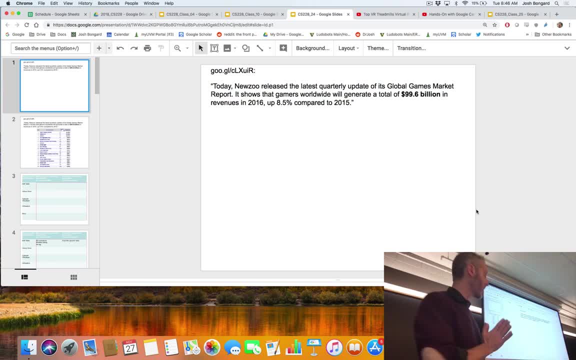 so, again, before we talk about video game, before we talk about virtual reality, to begin with let's start with computer games. it's pretty, pretty amazing phenomenon. back in 2016, games brought in a hundred billion dollars in revenues. compare that with Hollywood in the same year. so the most popular movie in 2016. 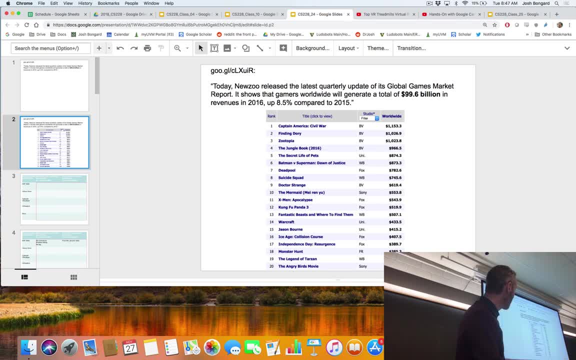 brought in 1.1 million, the next one 1 million if you sum the top 20 movies from 2016. it's nowhere near computer games. right there, it was a few years back, where revenues from computer games survived, and it's nowhere near computer games- right there, it was a few years. 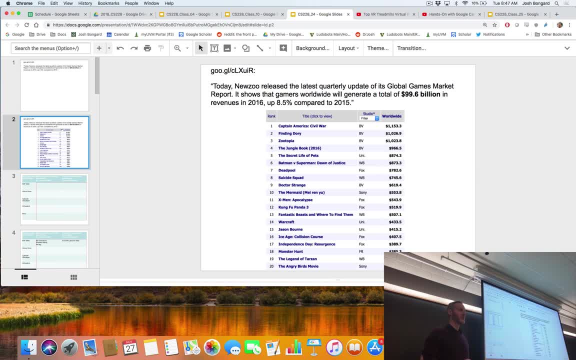 back where revenues from computer games survived and it's nowhere near computer past movies and now it's, I think, double. it's beyond that right. so there is something about computer games and this idea of engagement, losing yourself in the system that is increasingly attractive compared to our current. 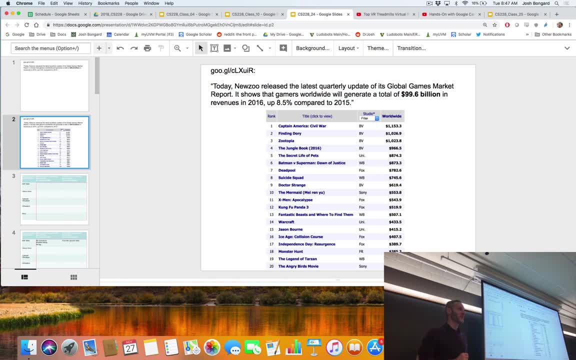 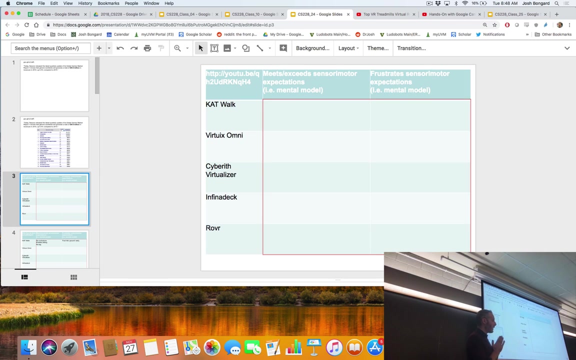 state-of-the-art system, or then state-of-the-art system for creating virtual world. it's pretty pretty amazing. yes, that's what is that? that is 1.1, 1.1 billion. Captain America brought in 1.1 billion. still not bad right, okay, okay. so we're gonna watch a minute of a video in a 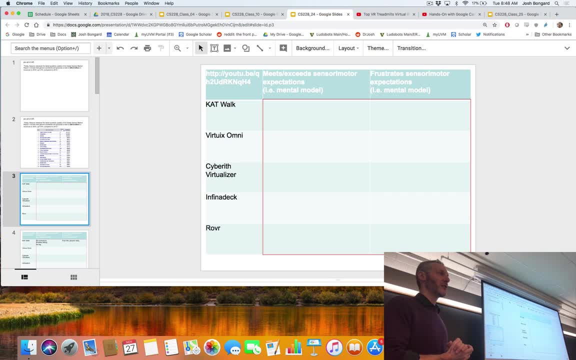 moment and we're gonna look in that video at five different VR systems, and these were sort of state-of-the-art prototypes in 2016, so they're already two years old when you watch this video. all five of these they're more or less promotional videos, so the demonstrators of these systems they're going to be. 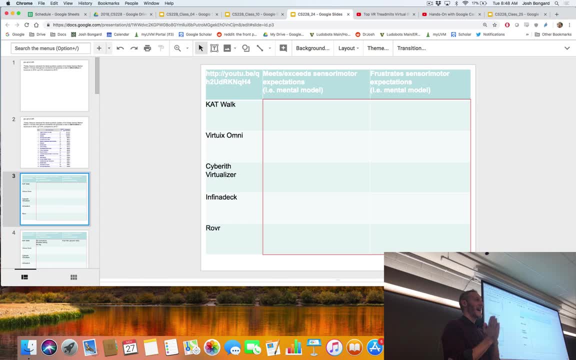 much more vocal about the advantages of these systems. they're not going to advertise the weaknesses of these systems. I want you to pay careful attention to these five systems and note down the pros and cons of these systems, specifically as they relate to which aspects of the users mental model do. 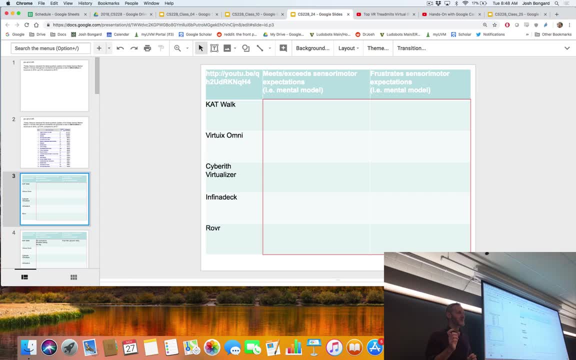 they meet and which aspects do they not meet? and which aspects do they not meet, which ones do they frustrate? and again, some of these are easier to see than others. so, for example, you'll see in all five of these that there is a goggle, and when the user moves their head, the scene moves in the opposite direction. in 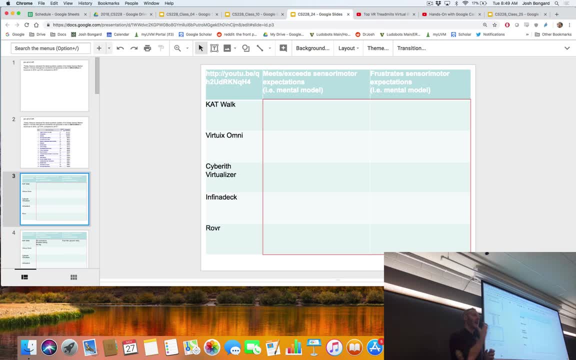 real time so that meets our expectation of head movement and movement of visual field. right that that makes sense, that one's easy. some of these systems try and capture other aspects that are more difficult to capture. So look particularly for those subtle aspects of sensor-motor coordination. 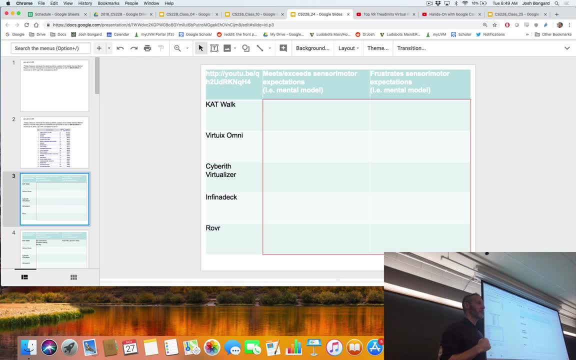 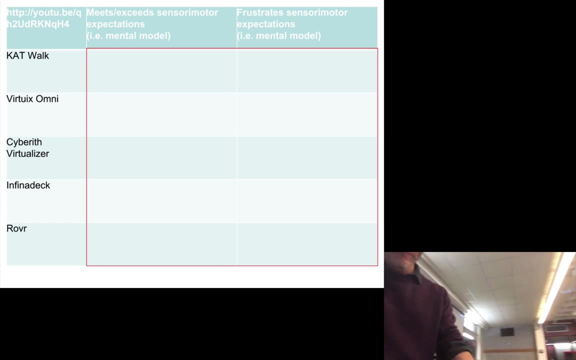 I push against the world and I expect how the world is going to push back. How many of those subtle expectations are met or frustrated? Those are the tricky ones to capture. Okay, Okay, I don't have any sound. Just bear with me for a second. 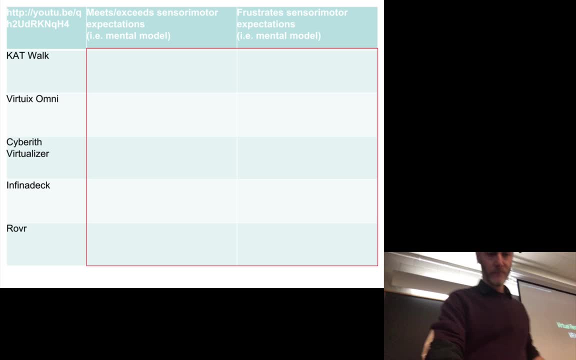 Let's switch those up here. Why run? Today, we're checking out VR treadmills that are either currently on the market or under development. These devices add locomotion to the VR experience, designed to increase immersion. Let's check them out. 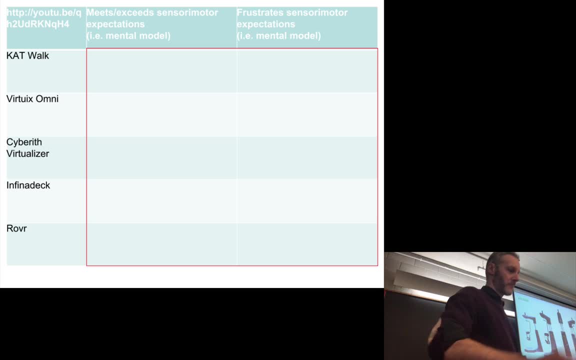 Catwalk is a new omnidirectional treadmill input device. The main problem Catwalk solves is to move within a small space in reality and achieve limitless and continuous movement in virtual reality. With its built-in and wearable sensors, you can literally walk, run backwards, jump, crouch. 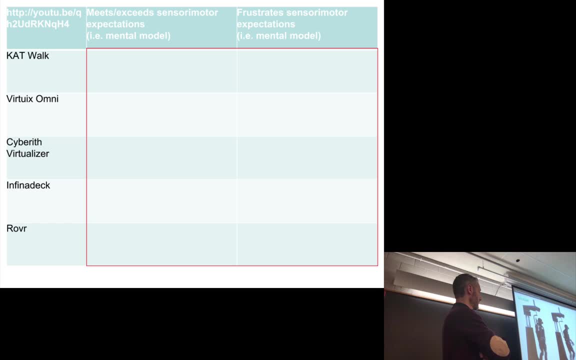 and sit in the virtual world. Different games call for different movements. Catwalk allows you to switch actions anytime you want. You can even sit down to drive or fly when a game requires it. We started the project since 2013, and we have made quite a bit of prototypes. 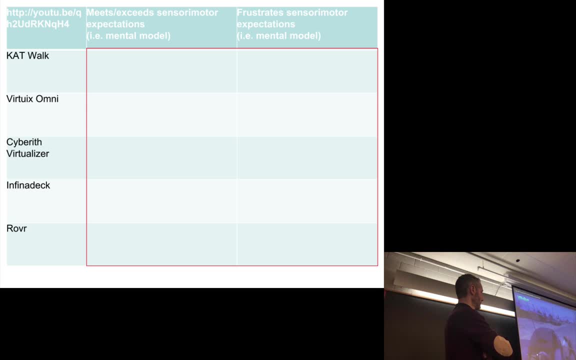 During developing and testing, we noticed that in many games you want to perform different actions with your arms and legs. It was annoying and disappointing if these movements are constrained And while in a virtual world you can't see the real one if there are devices near your arms. 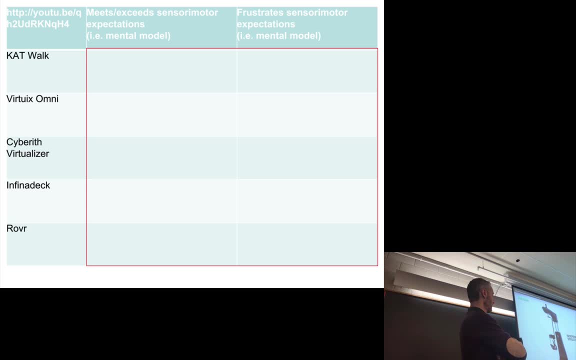 and legs. you may hit something or get hurt. The creative Catwalk app is a great way to get started. The Catwalk independent support structure and open construction set your arms and legs free First. it is very easy to get in Without a ring or column surrounding you. you can move freely and securely without constraint. 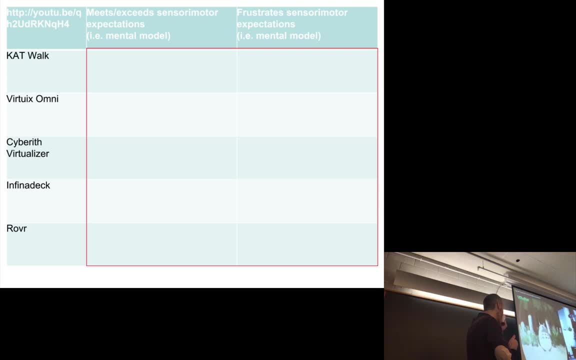 or worry about hitting anything. You can swing your arms naturally or put your hands to rest down by your sides, getting closer to a natural walk posture. Catwalk has not just simply removed the column and the ring. Our unique design can limit the horizontal moving range. 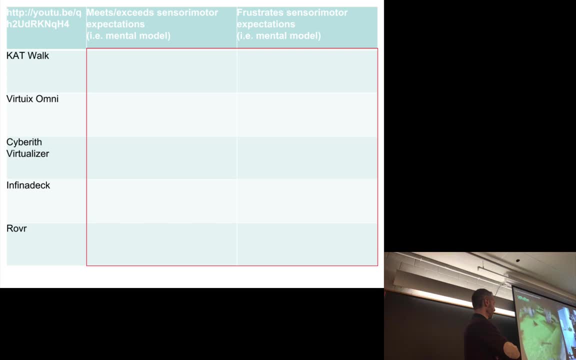 and control the vertical movement. It can automatically provide 35cm vertical moving range while jumping, crouching and sitting. Meanwhile, it can help users move back to center to adjust the position offset while walking, which can increase the sense of balance and safety. 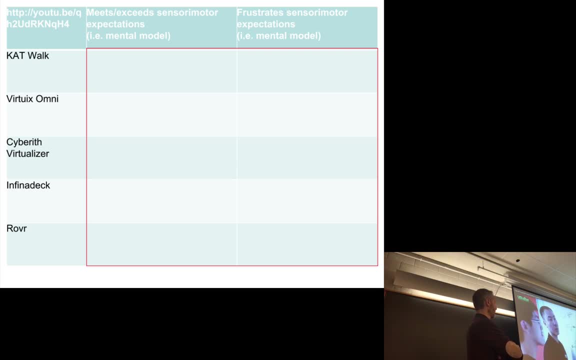 When we walk in real life, friction is what propels us forward. Frictionless walking is awkward like walking on ice, if you must pay attention to keep balance. Catwalk uses high-friction material surface and uses a coaxial movement. 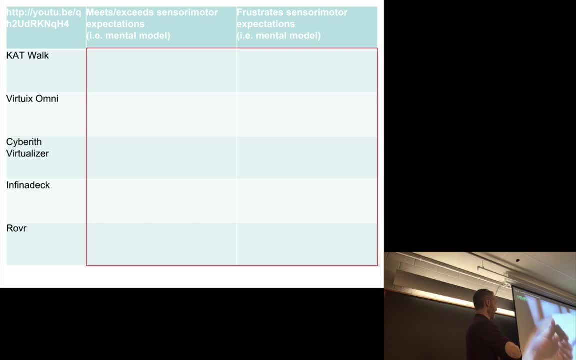 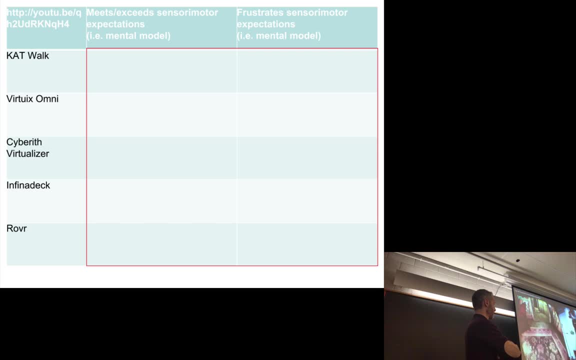 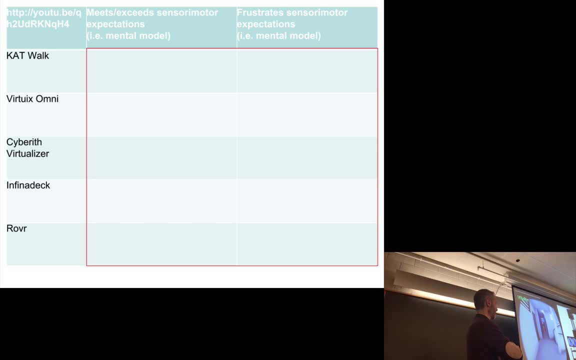 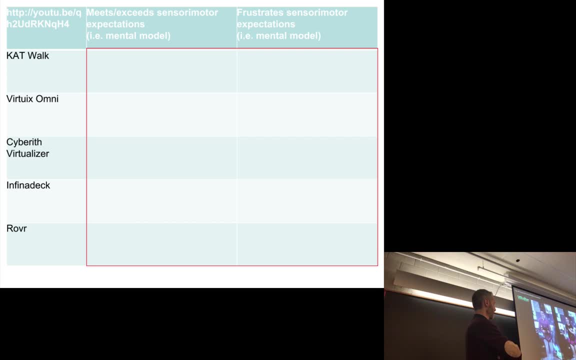 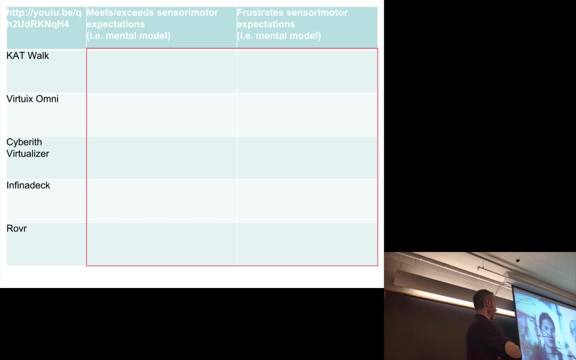 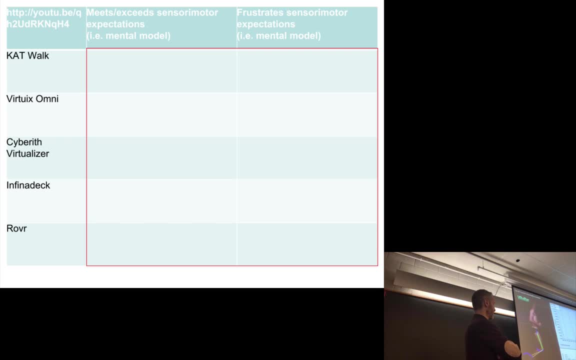 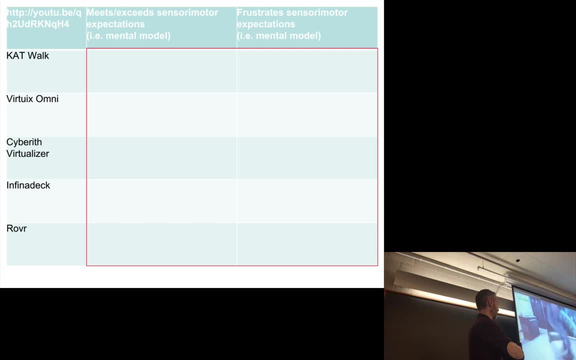 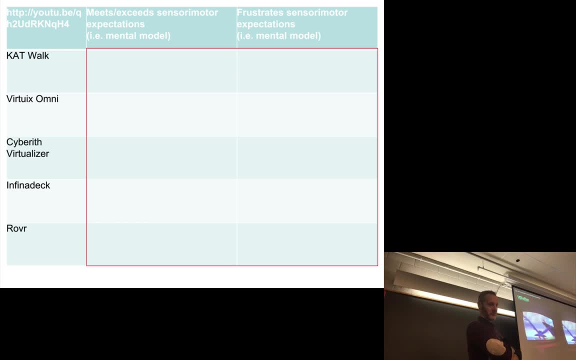 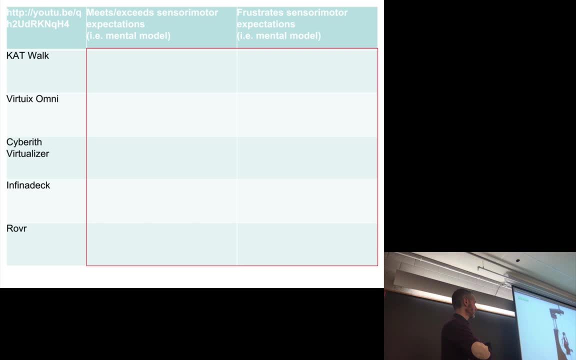 Catwalk uses high-friction material surface and uses a coaxial movement. Catwalk uses high-friction material surface and uses a coaxial movement. comfortable way- Just sit back and relax. Our software can transfer body motion to keyboard or gamepad. This means all the games with keyboard or gamepad support. 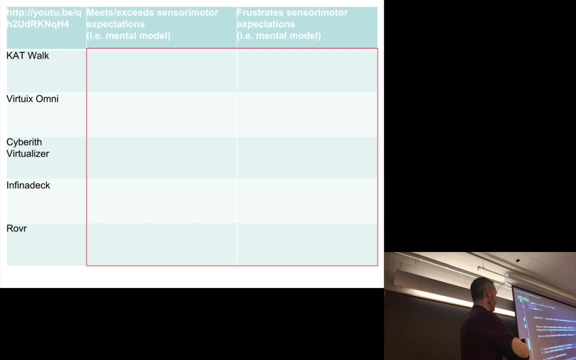 will be playable. We are also developing our own SDK and demo to achieve analog movement and independent walking and looking direction. The prototype you see here is kind of big. This was made to prove our brand new solution. We already have all the plans to make it smaller and lighter. 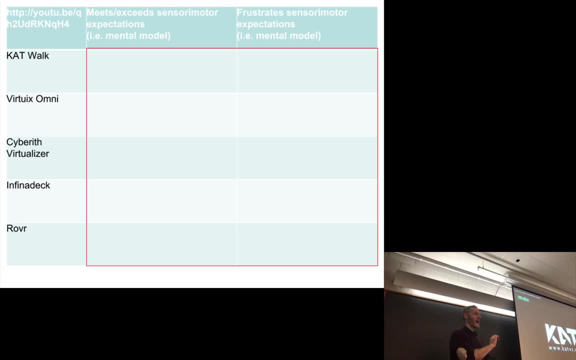 Okay, we'll see the others in a moment. What are some aspects of sensor motor coordination that are met and some that are frustrated here? Okay, so you can move in any direction and not bump into anything. That's good, So there's no obstructions. 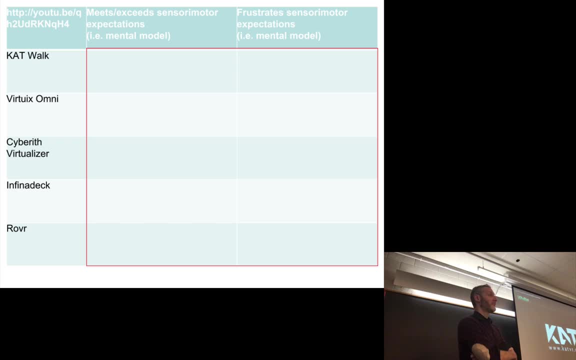 You don't have any. That's true, right, So there's just the, the goggles and the harness that you're wearing, So nothing directly detecting arm position or hand position. Yep, okay, There was a mention here that you can walk in any direction, Can you? 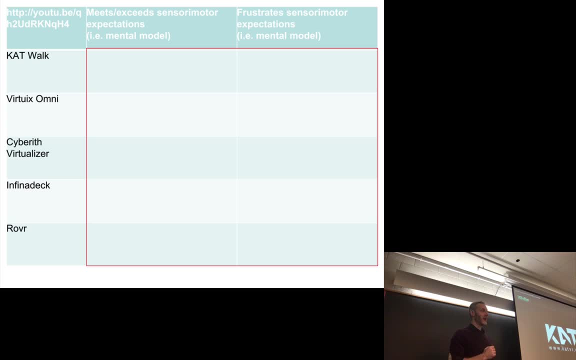 You can't walk backwards. You can't walk backwards. There's a limit to how much you can do there. Okay, possibly. So from what it looks like you can't actually like follow the step, Like you can't put one foot off of an edge and then fall, because that wouldn't. it doesn't go with the. 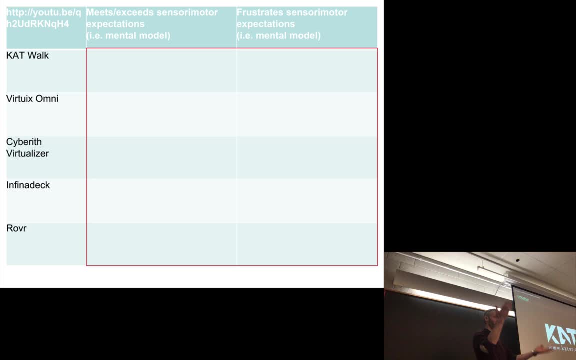 Right, So that's a good trade-off between safety and realism. right, So you can fall in the real world. but maybe not a good idea in VR. It seems like with the wheelset I don't have. It seems like with the wheelset I don't have. 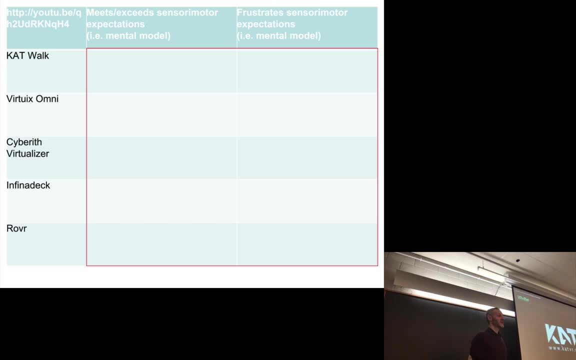 It seems like with the wheelset I don't have, So the wheels on the soles of the shoe. if you saw that in the video, right these high-friction rollers on the soles of these special shoes that you wear, so that when you step and place your foot in front of you and pull back towards you. 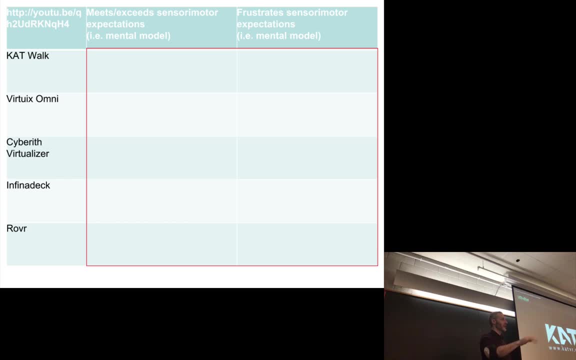 your foot, your leg feels resistance right, which is what happens in the real world. The sole of my foot- unless I'm on ice- holds still and my body rocks over my planted foot right. So you feel that according to this system, even though you are not moving forward. 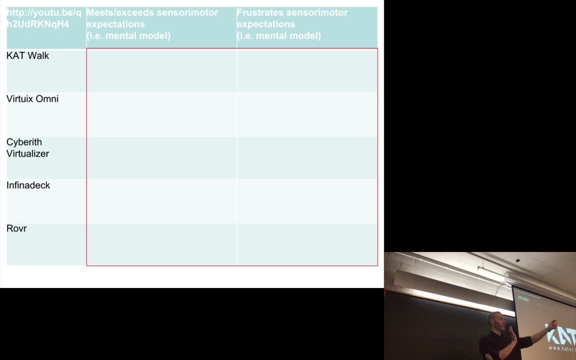 and putting your weight over your foot. it's the other way around. Your foot is rolling backwards towards you and your center of mass is staying in the same place. Makes sense, right? You want to try and keep the user more or less in the same place. 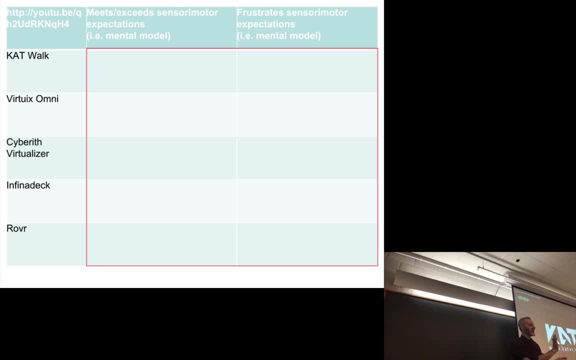 but it means certain movements- Motions like walking to the side- are not going to work in this system. Maybe that doesn't matter too much. You know- they mentioned that you can make a pivot movement when it's too far and it walks away at a museum guardrail or something and it stops there. 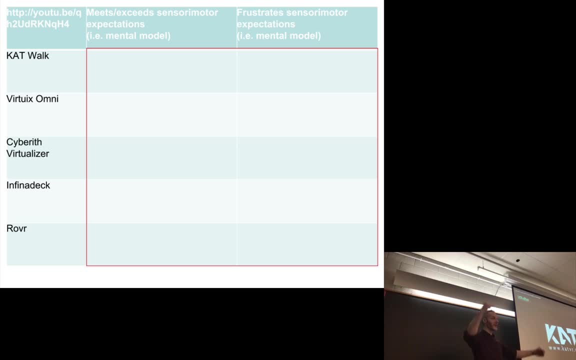 Absolutely right. So if in the virtual world there is a virtual barrier, the harness that you're wearing can enforce a physical version of it, right? So it feels like you've actually hit up against a barrier in the virtual. There's some more subtle interactions here that are also frustrated by this system. 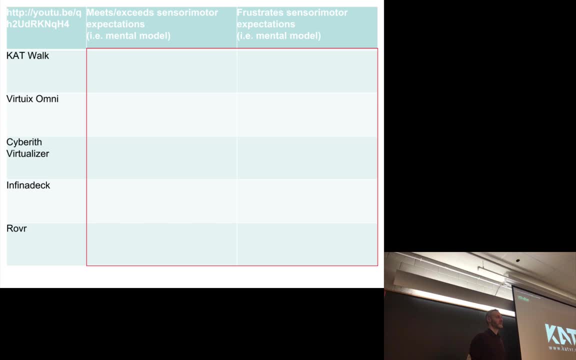 I don't know why you want to, but if you can roll or something, then you can do it right. I mean that's like a good one. but Right until we figure out the holodeck right, Actually, completely free movement is going to be tricky, That's fine. 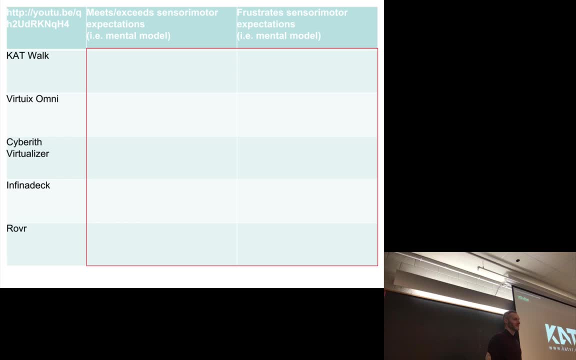 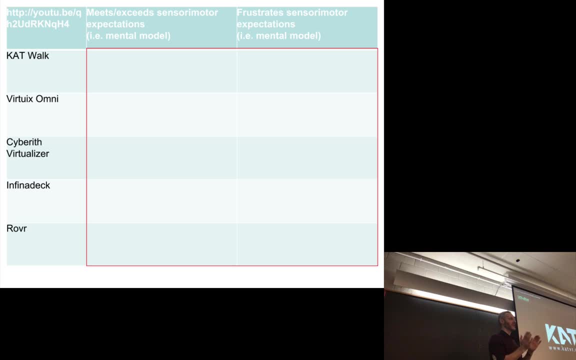 Let's go back to walking for a moment. You all have years and years of experience walking. As you walk- and you're probably not conscious of this- you will be after this class. what are the body cues that you're receiving as you walk that are frustrated by this system? 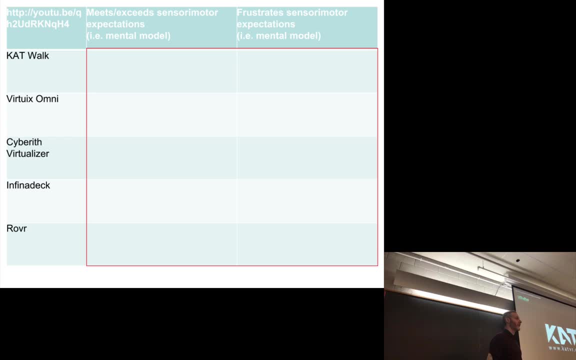 Air resistance, Air resistance- How? so You're actually taking a step in the real world? Yeah, You feel like air hitting your like face and your arms and stuff. Okay, yeah, that's a good point. Yeah, as you're moving through the world, there is a subtle flow of air. 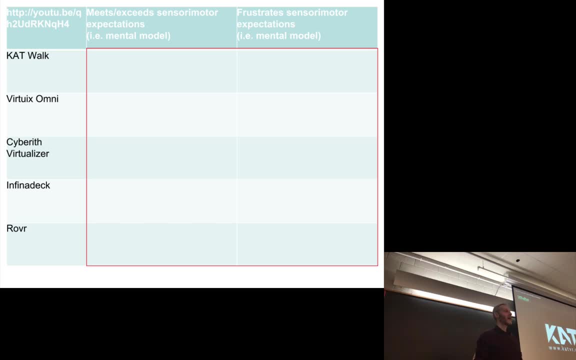 That's true? Yeah, maybe that's detectable. Your body is rocking back and forth, Absolutely so. your body is rocking forward and back, and you're wearing this harness, which is hard to see from this video, may or may not constrain that motion. 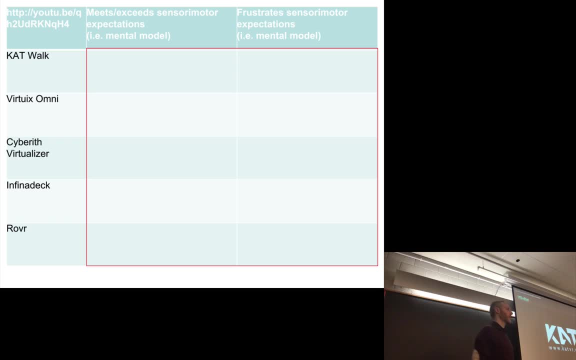 It doesn't look like you have anything for change and elevation, Change and elevation, Exactly, Exactly, As you walk along flat ground. what do you expect to sense as you do so, As you're walking uphill? what do you expect to experience? 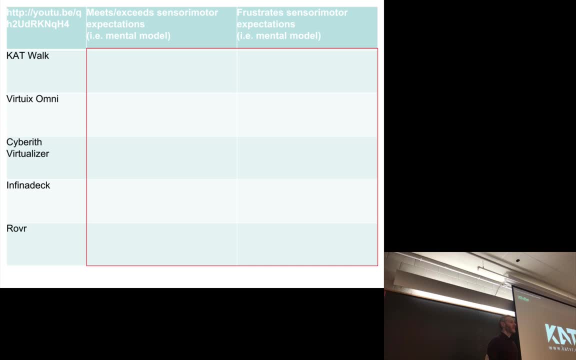 You change, kind of like, your center of gravity a little bit so you like can go forward, or Okay, yep, You feel the, You feel the incline right, and if you're walking up the side of this bowl, maybe people 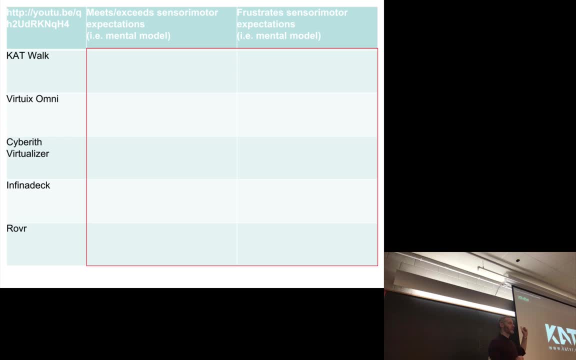 are rocking forward. Remember the cartoon I showed a few minutes ago: If I jumped up to somewhere higher, I would expect to land sooner than the time it took me to reach. like the, It's like I would jump and then I would reach the peak of my jump, and then I would. 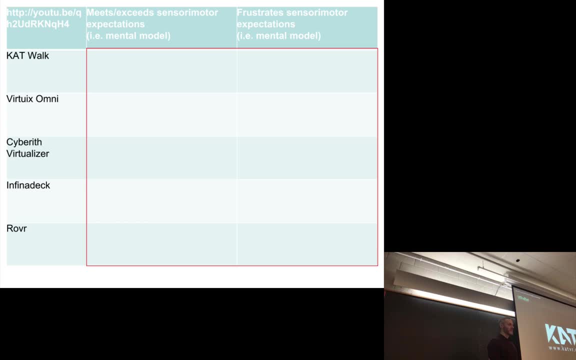 land somewhere higher up and I would expect that I'd take a shorter amount of time, but it won't Exactly So. there's an issue- There's a lot of issues here with timing in relation to locomotion right. So as you jump up onto a step or a block, you expect to feel 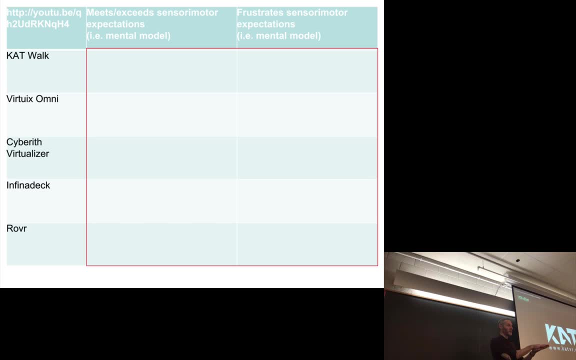 To expect to feel pressure on the soles of your feet earlier than if you jumped on flat ground. Okay, What about walking? Forget jumping for a moment. Walking on flat ground, walking uphill, walking downhill? Doesn't this device have kind of rims, the way you're walking around? 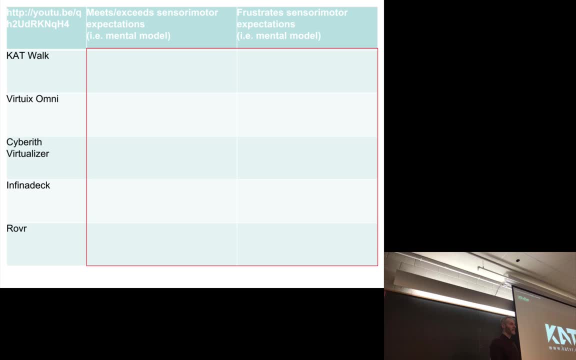 You're going to feel this all the time when you walk. The ground is flat, Absolutely So if you go back and watch this video, you'll see in most of the cases they're walking or running on flat ground, But in reality they're walking on flat ground. 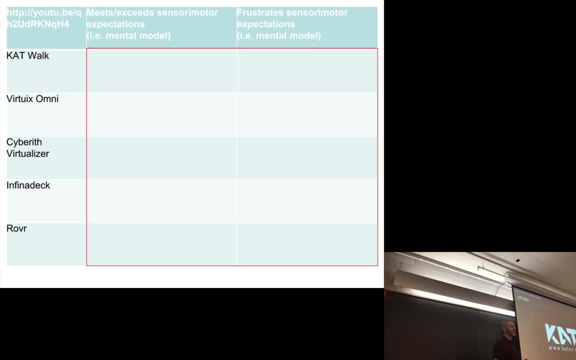 In reality, they're walking uphill all the time. right, They're taking a step and their foot is landing on the rim, so they're. It's like when you stumble on steps, Your expectation of when you're going to feel pressure is thrown off, and if you've ever 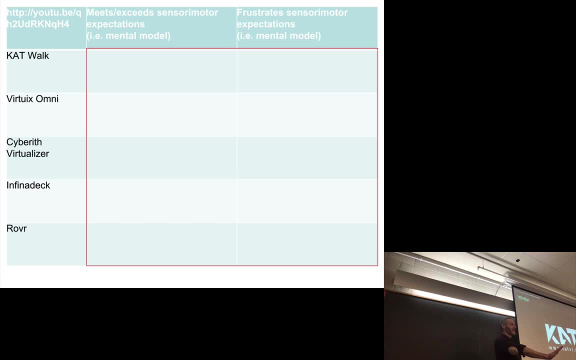 had that experience on stairs. it's very frightening, right. That's a pretty important signal when that particular expectation is frustrated. the timing in terms of football, I would imagine. I haven't tried this device myself. I would imagine it's a little scary at the beginning because you're not quite sure about 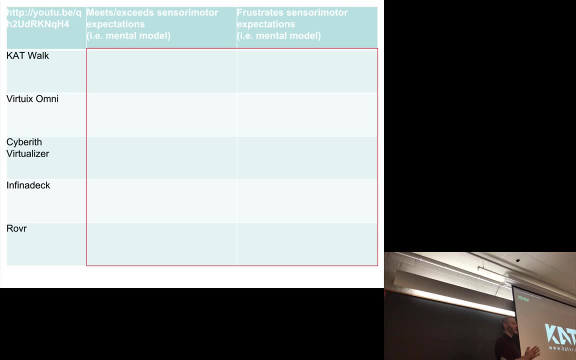 when you're going to step down. Now, again, the brain is pretty plastic. It probably adapts, but it's one of these examples of what makes VR so challenging. Okay, Okay, Okay, Okay, Okay, Okay Okay. 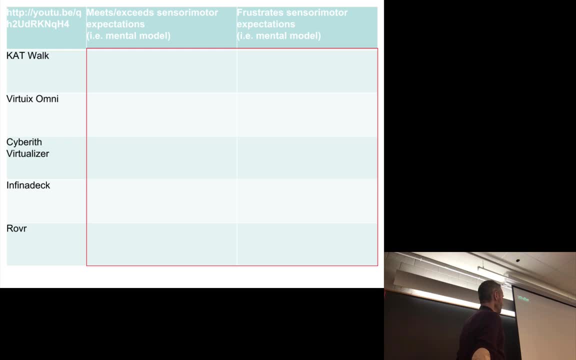 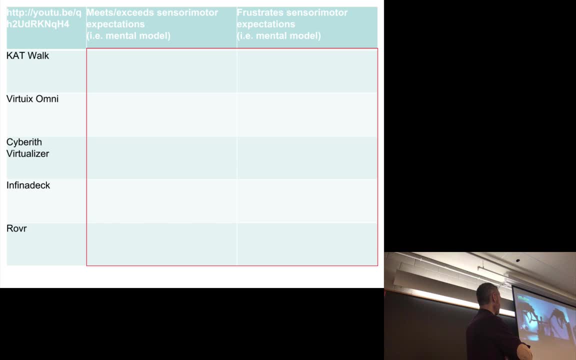 Yeah, Yeah, where games have always been trying to take you. they always talk about immersion and trying to actually put you in the game. well, you can't just do that with only a console, a controller and a tv. it is immersive, but you know, you're still sitting on a couch hopping on something like the omni. 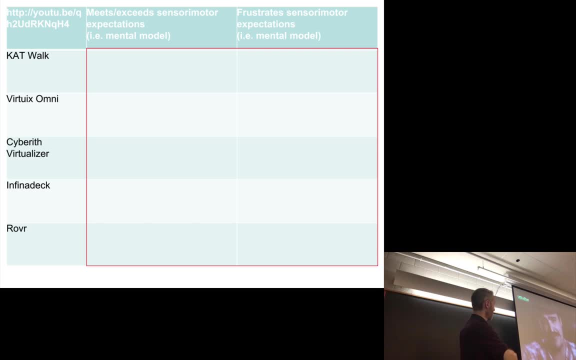 where it just it puts you in the game and you it's like you're suited up to get into the battle. i have a extremely bad problem motivating myself to do exercise. yeah, i broke a sweat in like that short amount of time. it's gonna get the heat turned up in here. i don't know getting to enjoy. 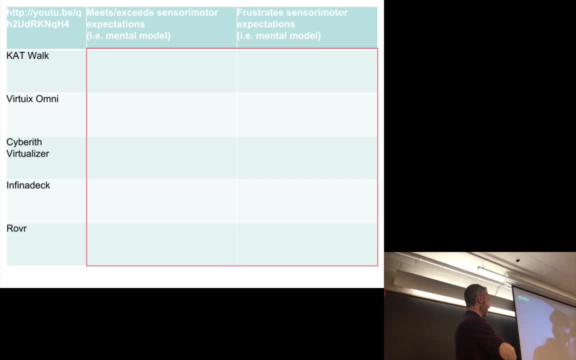 that physical interaction of running and moving and looking and not feel so detached from the world that you're playing in it's night and day. i have told people for years, if i could walk across skyrim i'd be more fit. and this is exactly that, that machine. i was like, oh my god, somebody actually. 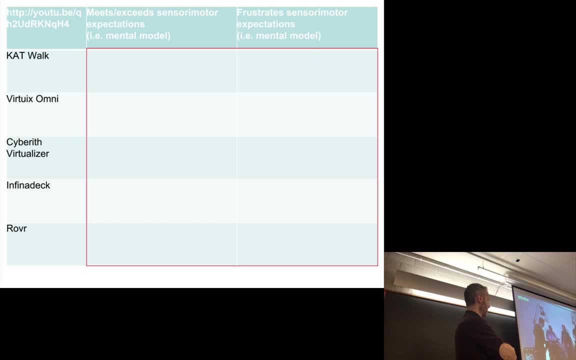 made that thing. i mean, i'm not much of a shooter, i just want to go explore a world, go running in, you know, a world full of dragons and magicians and whatever. the biggest thing right off the bat is the lack of sickness. so far, all of my experiences with seated vr- like i have motion 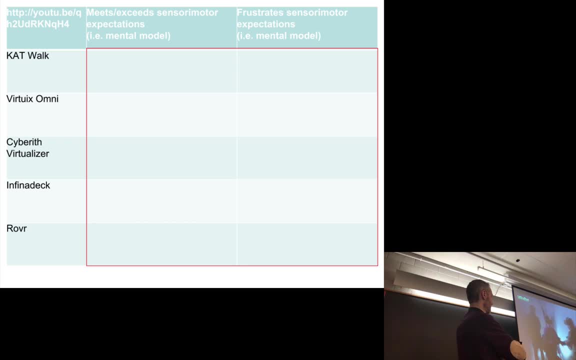 sickness stuff, and i had none of that here. what i loved about it is you're actually playing with people. the last demo i tried was single player and you kind of walked through this corridor, whereas this one was a little bit more wild because i had a partner in there right next with me. 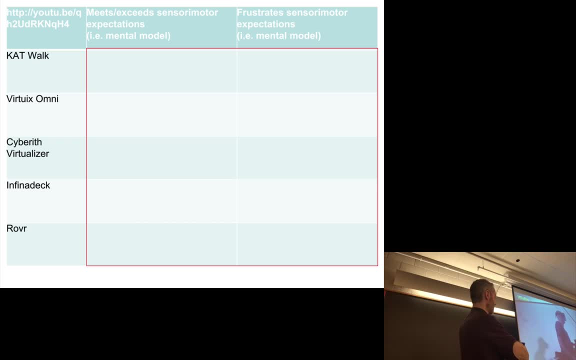 when the bad guys get close to you, you instinctively, like you move your body away from them. you react. my head moved and it moved and my whole body went with it and it was cool i could have this in my living room with my rock band equipment and i think that's really exciting. 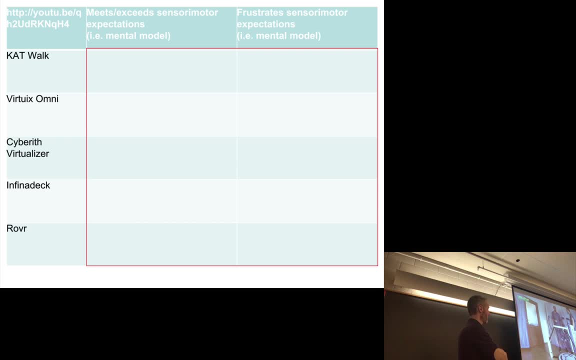 the virtualizer consists of three main parts: the bass blade with a low friction surface, the pillars and the ring construction. there are linear guards in the pillars that allow for smooth and quiet vertical movements. this is necessary for crouching and jumping, and in addition to that, the ring construction allows the user to turn around. 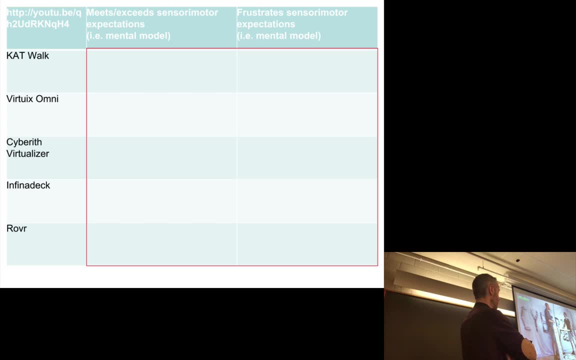 and rotate 360 degrees. we found that rotating inside of the second prototype wasn't as smooth as we wanted it to be, so we decided to improve the mechanism of the ring construction. furthermore, we also refined the sensor system that detects the rotation of the user. we have also changed the linear guide system inside the pillars, which is now smoother more. 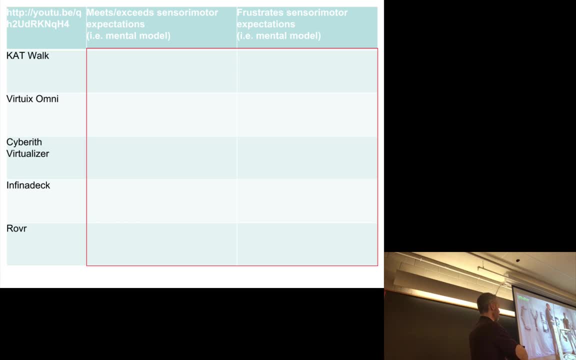 quiet and more durable. on top of that, the new system is lighter than the previous one, so we have saved some weight, okay. another major improvement is the material that we use now on the base plate. for us, it is very important to have natural walking and running inside the device, so the friction coefficient is now on a level which is ideal for natural movements. 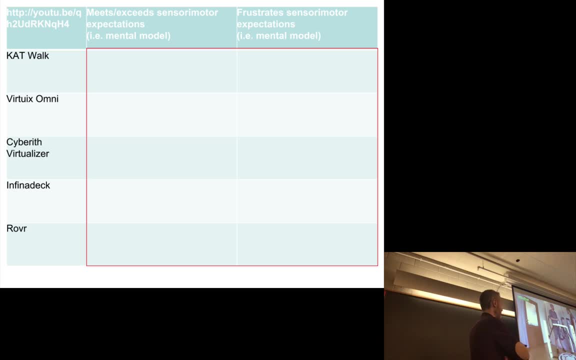 when we started developing the virtualizer, we made some experiments with different shapes and also made a motion analysis in the laboratory. we have also tested the different shapes in action and we have realized that the flat base delivers the best immersion. now, if you use a bowl shape, 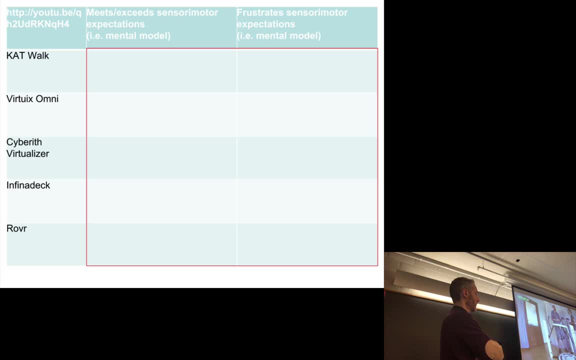 your feet will touch the slope of the bowl earlier than you would expect, creating a discrepancy between what you see and what you feel. this breaks immersion and pulls you back into the, into reality. stability is very important for us, so we decided to use three pillars instead of two, or just one. 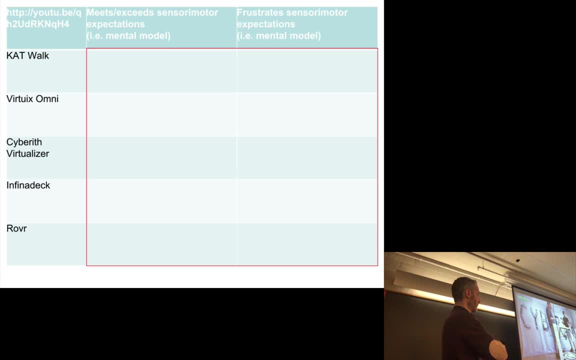 the reason is that three pillars absorb the forces of the momentum caused by the user, rather than two or just one pillar, and since you're able to sit down in the virtualizer, you can come from two or just one pillar. you can try to jump in one of the rows. 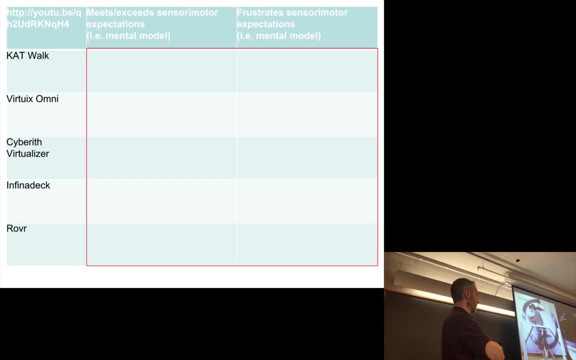 you have to make sure that the construction supports the user's weight. speaking of the setting function, obviously you have to be fixated inside the ring and to perform moves like jumping and crouching, and also for us to sit down. does the user have to carry all the weight? 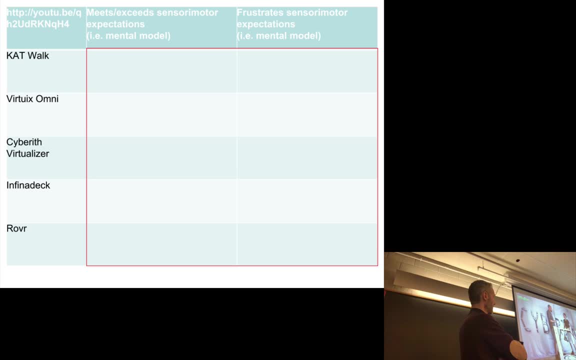 of the ring construction as well while he does so, or do you have a solution for that one of the ring construction, so the user doesn't have to carry the weight and doesn't feel anything of the reconstruction? okay, so one thing you notice about the new prototype is that you've constructed 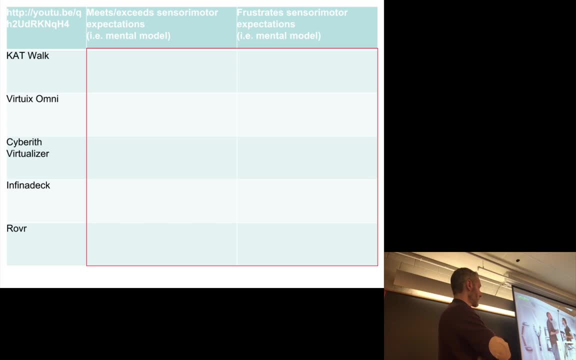 a black bar which is hanging above your head. now could you maybe explain the reason for it being there, sure? yes, we call this black bar vr, and it is constructed because of head mounted displays and earphones which are wired okay, so you can guide the cables all the way ahead and don't. 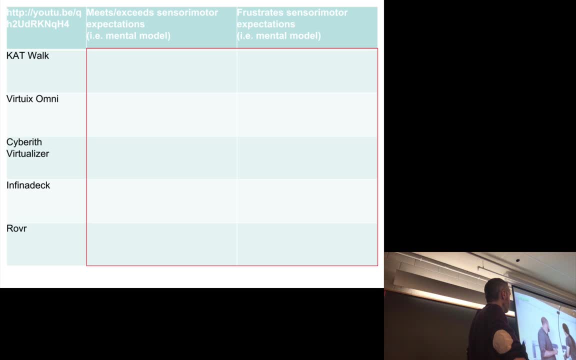 get disturbed in the virtual world. okay, and it is decided that way that you can still aim upwards without tossing against it. i see, so it's all completely unrestricted, absolutely okay. i see, okay, i think that's enough for now. thank you for taking your time off to show us the virtualizer. 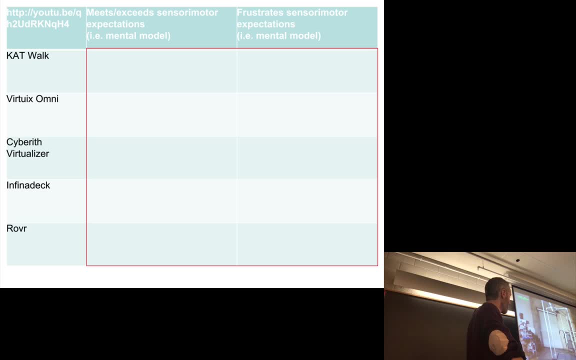 welcome to infinideck, a true omni-directional treadmill. infinideck uses motorized components and a simple belt connected to a sensor to track and respond to your movements in real time. infinideck's belt has multiple bands that change direction, allowing you to go in any direction at your own pace. 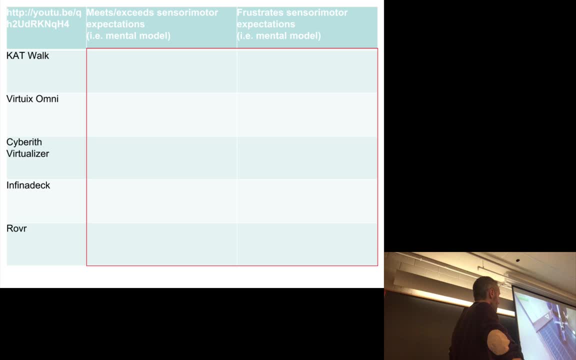 freeing you to explore your virtual reality environment naturally and safely. infinideck revolutionizes virtual reality movement, giving you the ability to quickly change pace, stop and go, crouch and pivot, providing a truly immersive experience. with our technology, you can feel like part of your favorite game or jog through exotic countryside while at the gym. 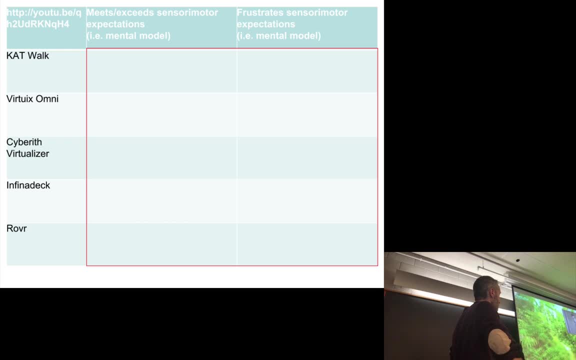 infinideck makes the future possible today. imagine training simulations that prepare you for urban warfare, let you practice tactics on foreign terrain or even walk beneath the stars of another world. infinideck's omnidirectional treadmill technology makes it possible for you to be fully. 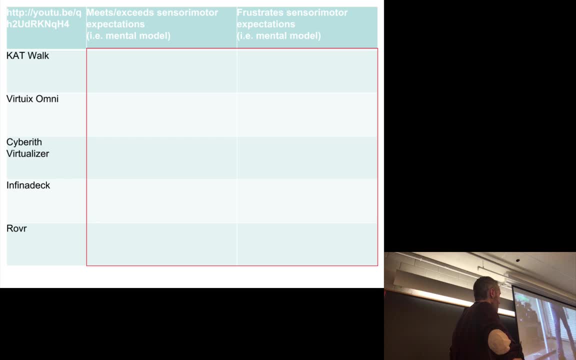 engaged in the vr world while keeping you safely in the center of the treadmill. Need to save money signing up as a member of the finideck team? Invinible- please move your tiara. please click here to help your team keep more footage and 20 public images available to visitors. 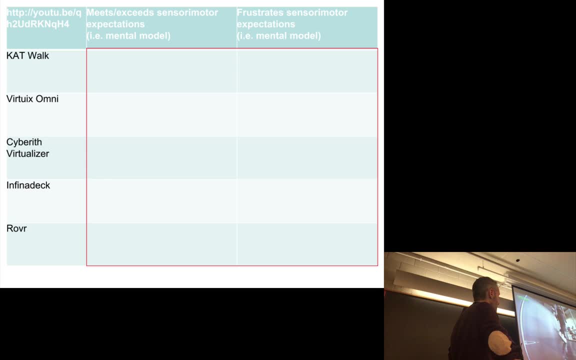 formation plus motivation for future transformations into your own life. and Granny running a shootout for her master's degree. Thank you, Thank you. Last one, Mm-mm. Sometimes simple is best. Mm-mm, Mm-mm. Okay, I think you get the idea. 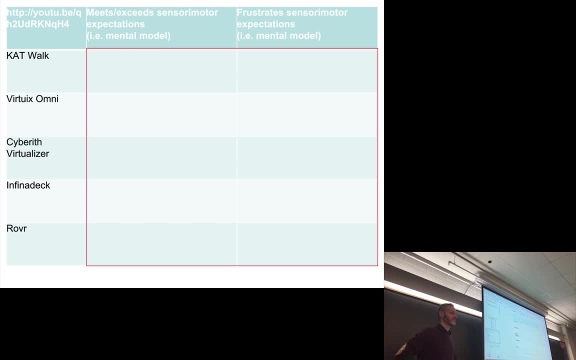 Okay, pros and cons They all, like I mean, now that I see all of them, the illusion of free movement would really be broken when you walk up to something and try to touch it. If you walk up to something and try, 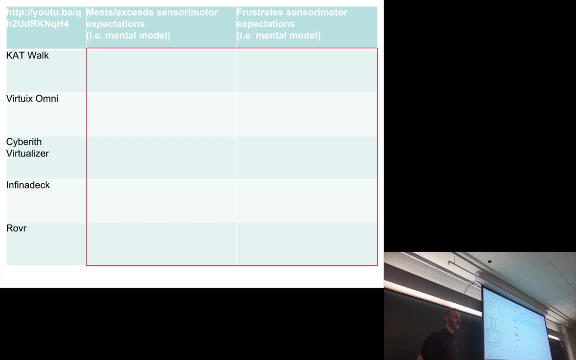 and touch it. it's not there. Why would it be broken? What's missing? Like the guy with the um walking around that, like the with the infinite deck and you like walk up to one of those posts and he was like reaching out with his like. 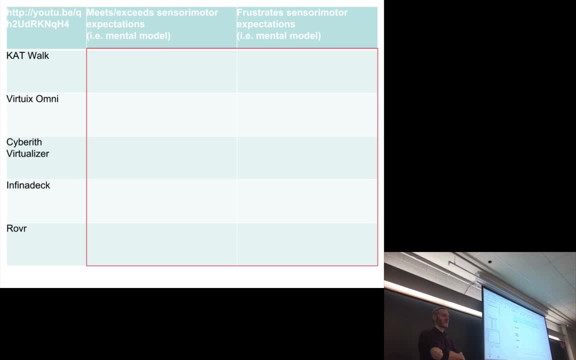 controller or whatever, Like you reached out and you tried to act and you like, touched, put your hand where you thought that that would be, you would expect to meet some resistance, but instead you're just waving your hand around. If you were to reach out and try and touch an object. 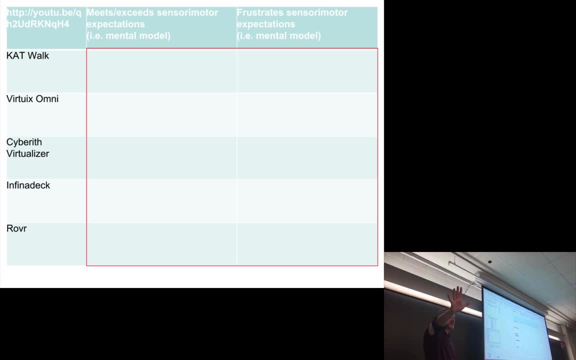 in the virtual world, you would expect to feel resistance, but of course, in the real world there's nothing there. How might we deal with that? Oh, do you have an idea about that? Let's stick, go ahead. Um. 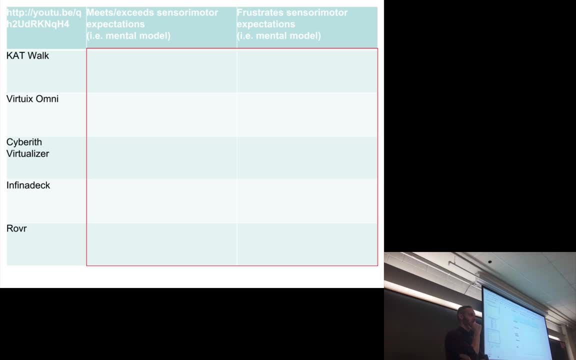 I don't know the point, but I don't think there's any kind of, for the moment, able to um walk into it, because it's not as much as I expected. but So of course there's different components. 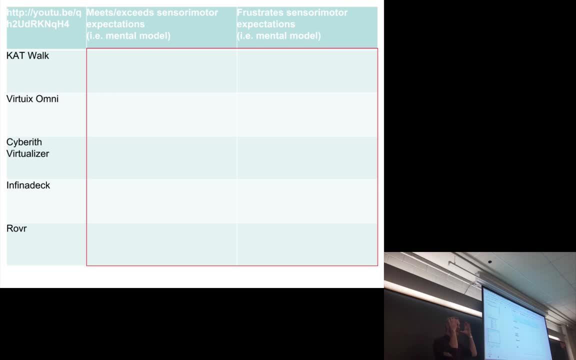 There's different components here, right? So VR systems are meant to be modular, so first of all was the goggles to deal with sensor motion and vision. We're primarily visual creatures so, again, not surprisingly, that was what was tackled first. 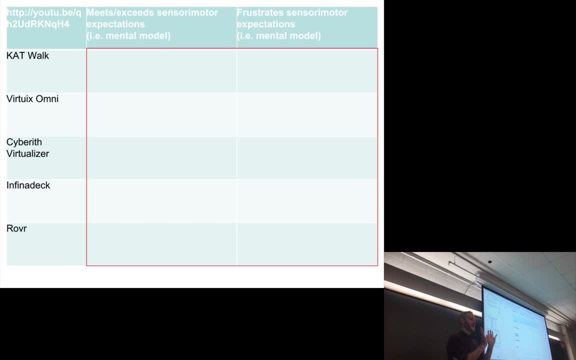 That technology is reaching perfection, more or less. Next is walking. We are mobile creatures right Then. the next frontier is reaching grasping manipulation, so we can create VR gloves. How are those gonna help us? If you have like haptic feedback with gloves? 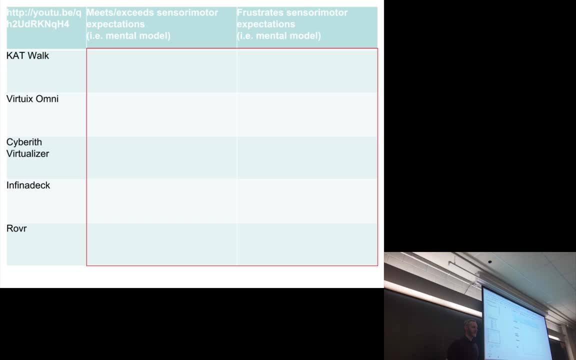 then you can feel resistance or pressure when you reach out and touch things. Absolutely so we could have haptic resistance. we could have special gloves that provide vibration, perhaps to give a signal of resistance. There isn't anything yet that's going to physically. 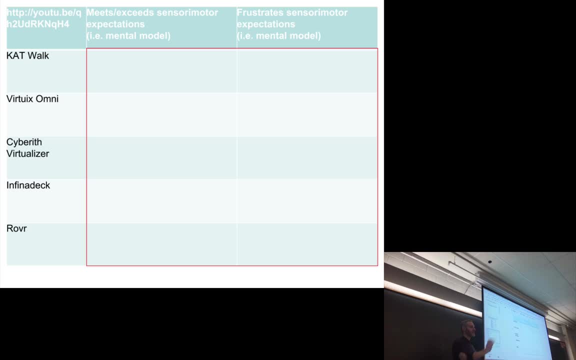 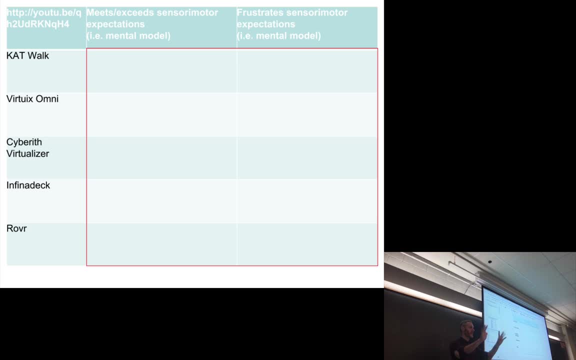 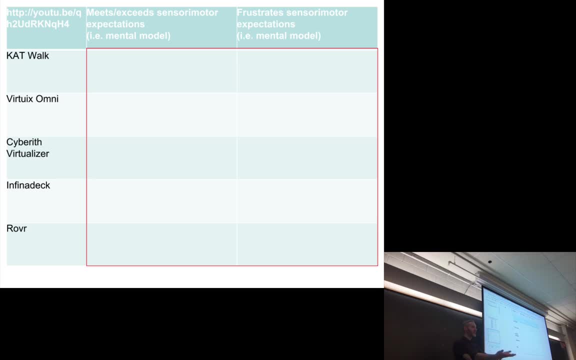 Ultra haptics, Ultra haptics, Exactly. You remember that system that was producing? that was producing ultrasonic beams from above. that was producing ultrasonic beams from above and when they met at certain positions in three-dimensional space, those waves would produce positive interference. 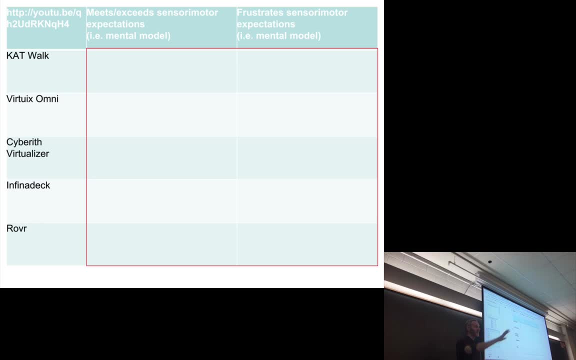 and increase the resistance there and you can actually feel it in the air. It feels like you're touching a virtual object. It feels like you're touching a virtual object. Imagine if you were to connect ultra haptics with a goggle and treadmill system. you could start to approach manipulation. 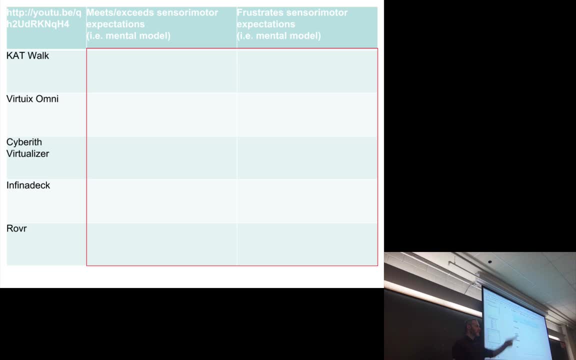 But again, manipulation is tricky. I saw a problem with the Infinideck where there was movement after you stopped moving. So also when the individual crouched, the treadmill moved a little bit, Exactly. So Infinideck has an obvious advantage, which is that you're actually moving right. 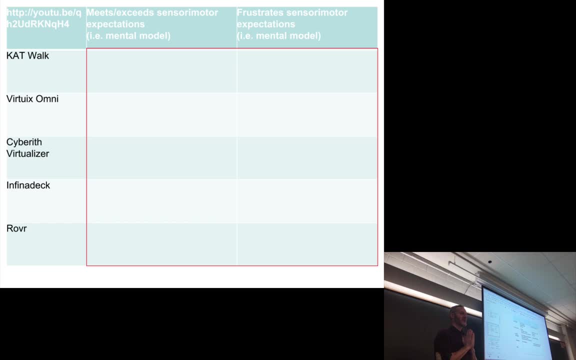 In the other four systems, your center of mass stays where it is. You put your foot out there and pull your foot back towards you, which is not what happens in reality. If you're on a treadmill, you are free to move your center of mass in a certain direction. 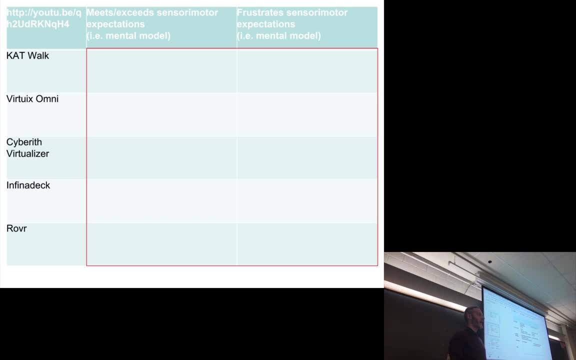 And then the treadmill under. you will pull your whole body back to origin. A great advantage, but it comes with a cost, which is the lag. You feel that motion of the treadmill slightly after you initiated the motion. That's an interesting idea, right? 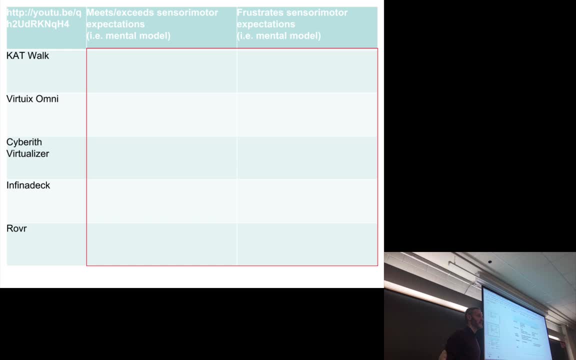 So these haven't tackled incline or decline yet They could. Let's focus on the treadmill for a moment. This is an interesting case With the treadmill: like so you didn't have to shift your center of gravity, but all of them- it looked like they were still leaning against the resistance of the thing that was holding them in place. 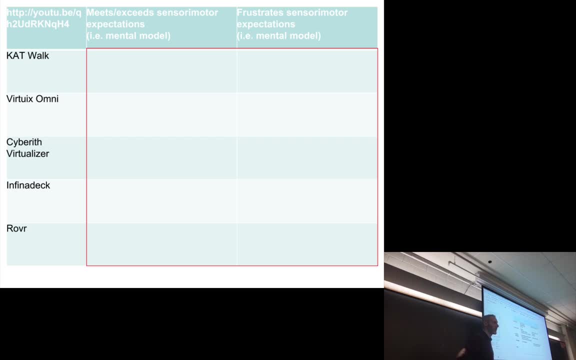 Okay, so maybe there's a little bit of. there's some complications there with the rig that they're wearing. Let's forget that for a moment and let's focus just on the treadmill. Let's take what we've learned in HCI about packed analysis. 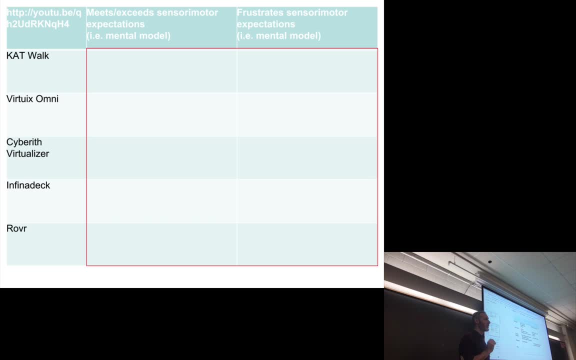 Let's think about physical context. In this case we're thinking about physical context of moving. A human walker is walking around in the physical world. They're giving off lots of cues about how they walk. We need to detect those cues. We need to sense that, send those signals to the treadmill. 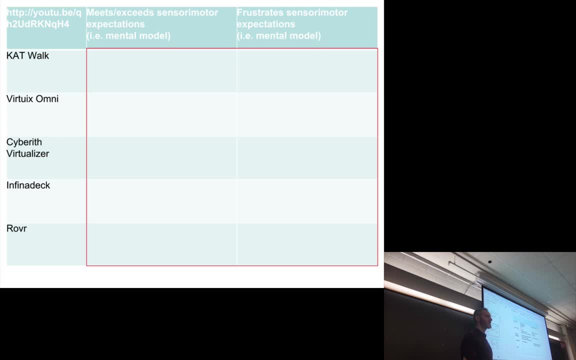 and get the treadmill to move in the right direction at the right time. There's always going to be a lag, but maybe we can get that lag small enough that it's not detectable to the mental models that most people have when they're walking. 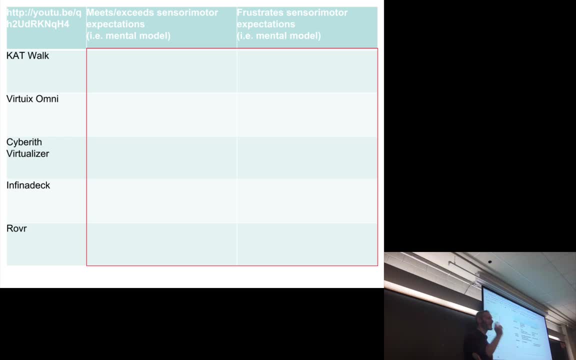 There's still a lag in goggles, but it's low enough now that for most people, they cannot detect it and they do not get motion sickness when they're wearing VR goggles. What are the cues that a human gives off when they're walking about, where they're going and at what speed? 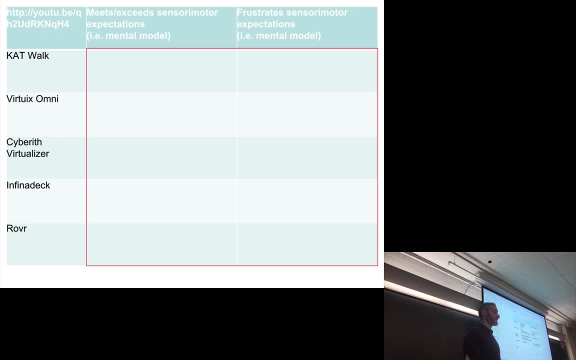 Angle of the head, angle of the hips. What about angle of the head? tells you where the person is about to walk. Normally, you look where you're going to go. Physical context, right. Most of us we turn and look. 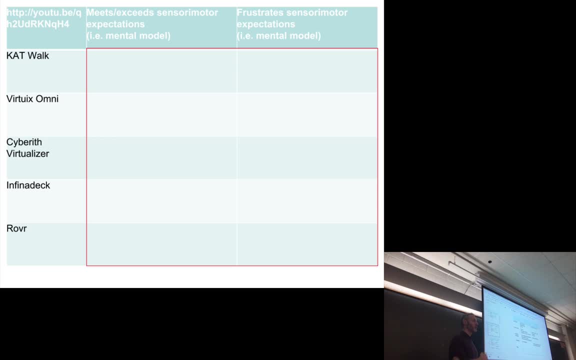 If we're going to change direction, we turn our heads before we turn. We could take head motion data which we're getting from the goggles and use that to improve the response of the treadmill. What else, What other signals are coming in about where the person is about to go? 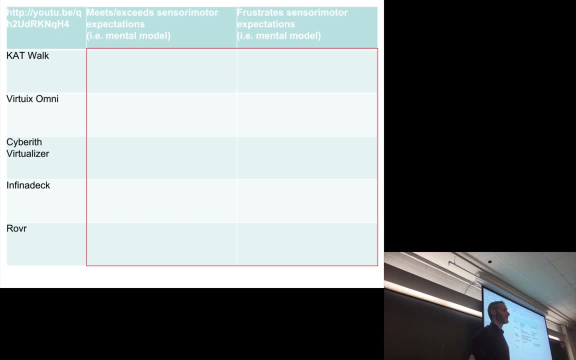 If you have a treadmill, it's probably running faster. If you don't have a treadmill, it's probably running faster. The treadmill, the system, may be able to support running. That may be a functionality you want to try and capture: Challenging, because now you've got high-speed motion. 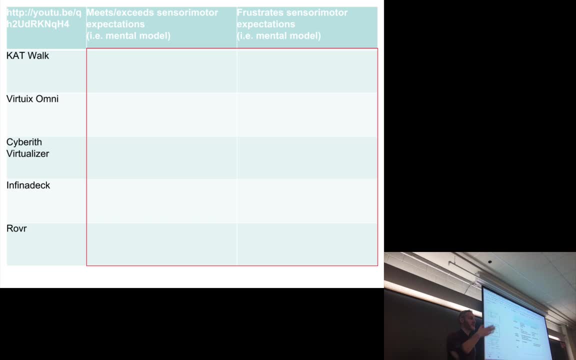 But there are unique cues that the person is preparing to transition from walk to jog or trot or run, Looking down and shifting weight a little bit forward. Assuming that again from the harness we're getting information about body posture, we may start to ratchet up the speed of the treadmill. 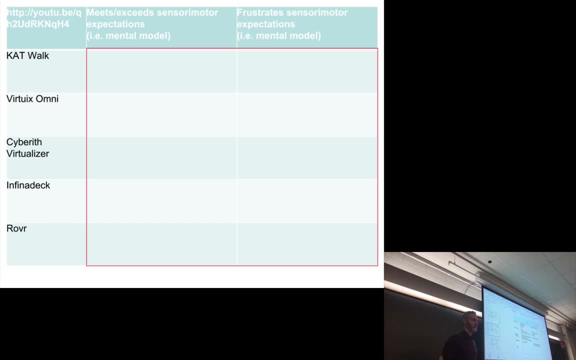 because the person is starting to accelerate. Assuming that there is pressure sensors on the bottom, like with the other ones, then you could kind of see how they're distributing the weight on their feet. Absolutely The relative pressure in the soles of the feet. 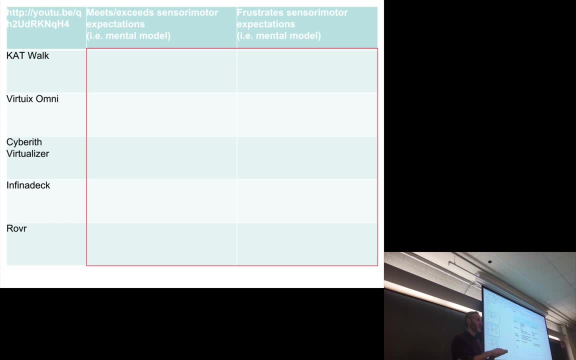 where pressure is on the soles of the feet is very indicative about twisting, turning, shifting weight. I'm about to jump, I'm about to crouch, I'm about to walk, I'm about to run, I'm about to stop. 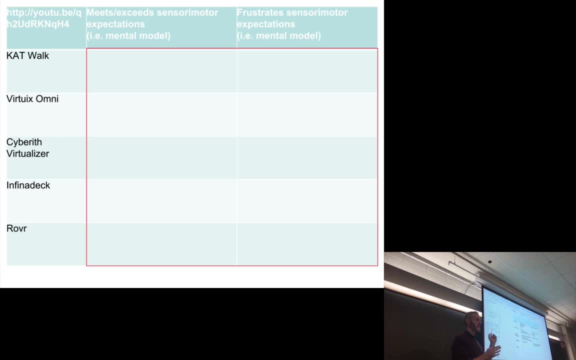 And so on. How does the treadmill itself work? The mechanics, How is it omnidirectional? There's one big belt, right? There's one global belt that is moving in one direction. We'll call it the X direction, right? 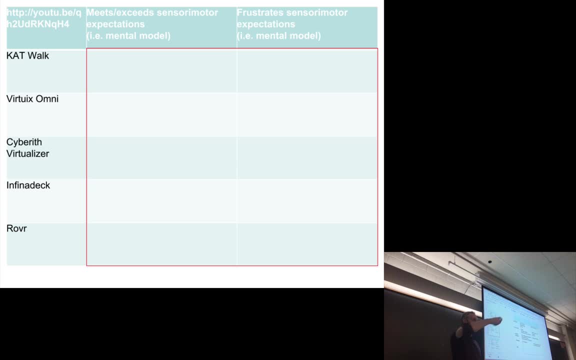 And the belt of that large treadmill is made up of a series of smaller belts which are moving orthogonally. Let's call that the Y direction- And each of those individual treads- if you go back and watch the video, can be moved at different velocities. 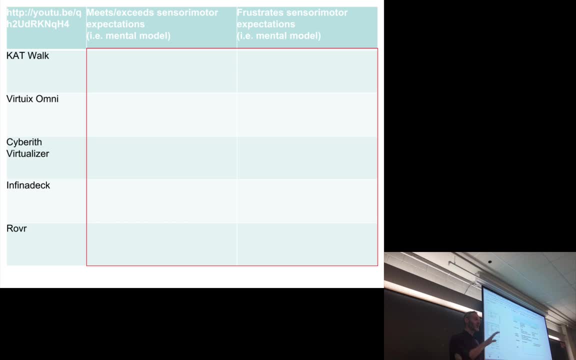 So it's not a uniform motion, which is good, because again you can just move where the treadmill can move, just where the person's foot is. But again the real world doesn't quite know how to work that way. Kind of an interesting mechanical system. 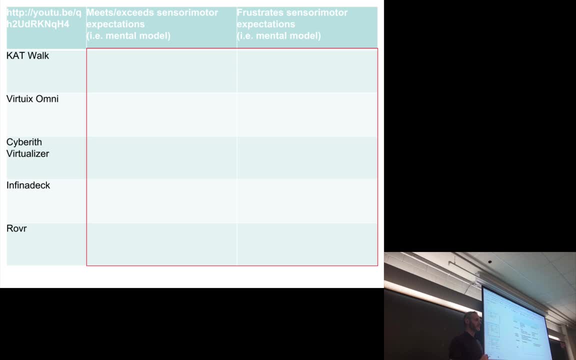 and then also interesting from an HCI point of view, The direction that they're moving. you mean, Yeah, Yeah, Tricky, Yeah, Absolutely So obviously a big, big challenge here. You can imagine massive user testing and all the different ways that people 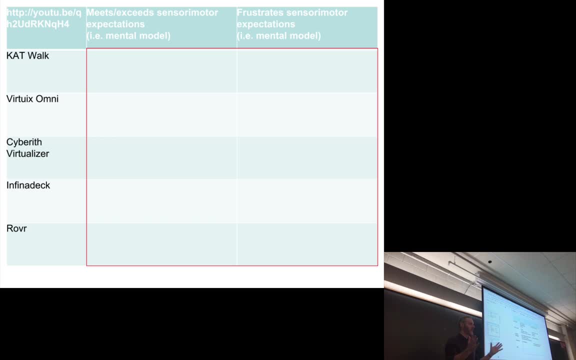 might move through a virtual world. You've got a massive amount of training data. There's a very interesting machine learning problem to be solved here, Given the current head position, body posture, pressure from the feet, sensor data coming back from the harness. 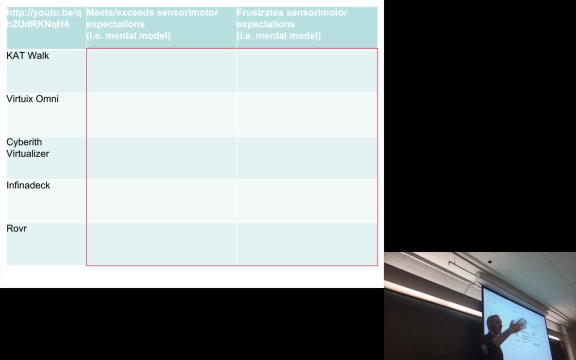 what direction and speed is the user going to move in? the next tenth of a second second, two seconds from now, and so on? Not an easy thing to do, but maybe not impossible. Okay, So I mentioned some of the other ones here. 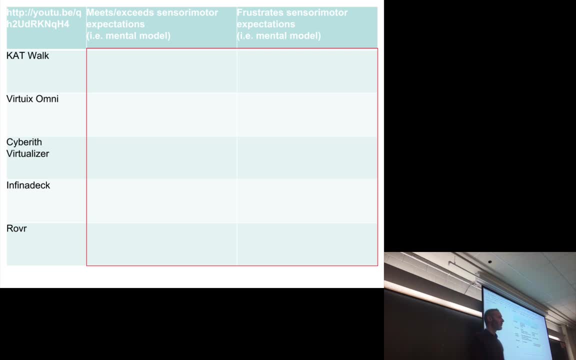 I mentioned passing motion sickness. Anyone try any of the earlier goggles? No, Okay. So why do people get motion sickness with goggles? What's the problem here, When your brain tells you that you're not moving, but then your eyes are telling you? 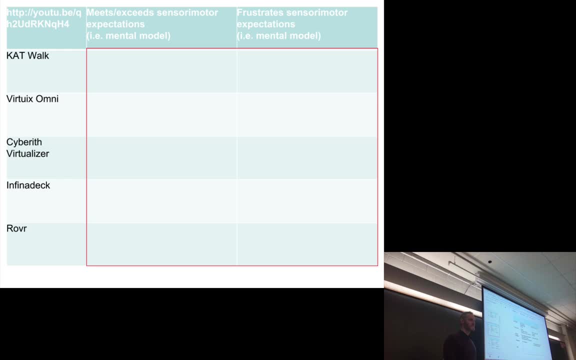 that you are moving, or vice versa, then it's. you know, your body doesn't like it. Your body doesn't like it. Same reason why some of us get car sick. right, Because it's not something that our brains were evolved to deal with. 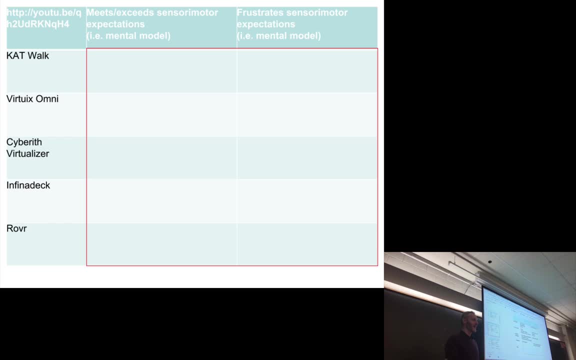 Our ancient ancestors never had to deal with treadmills and moving cars and so on. right When I move, the rest of the world moves. Typically, the rest of the world is not moving when I'm stationary or when I feel that I'm. 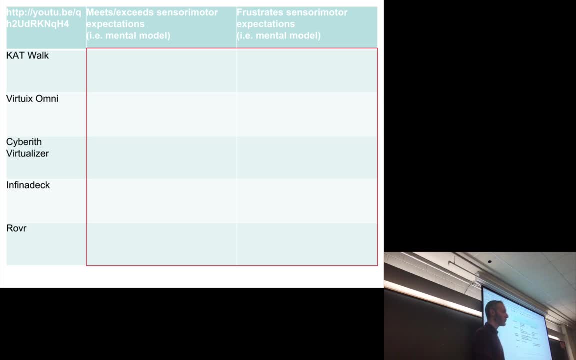 stationary. Okay, What about the last one here? Roper: Simpler design Pros and cons. It was simpler. One of the cons is that, like it wasn't really, we weren't really walking, it was more like a shuffle. 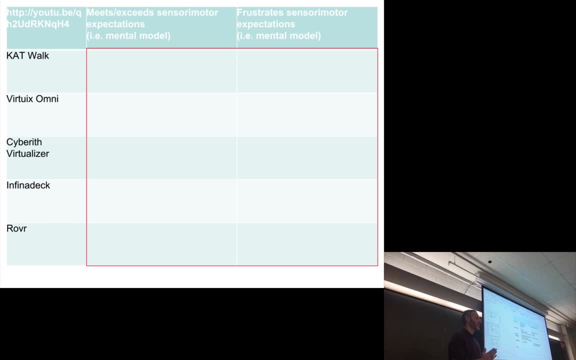 Right, Right. And again. for a lot of users, maybe that's good enough, right We're? we don't need to create a perfect, you know, we don't need to create a perfect illusion. It depends on what we're we're trying to do. 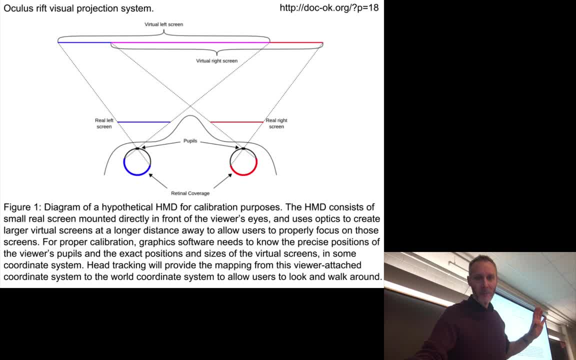 Okay, Let's, let's move on. Let's talk now about the goggles themselves. Again, this is more or less been solved, but kind of an interesting HCI problem as well. We need to again think about physical context and physiology of the visual system. 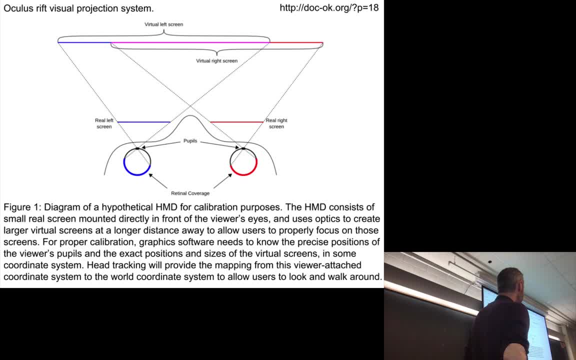 So here's a diagram of a hypothetical head-mounted display, And this is for calibrating head-mounted display. Most goggles have a left screen and a right screen, but because, again, physical context, we're wearing the goggles, those screens are very, very close to the eyes. 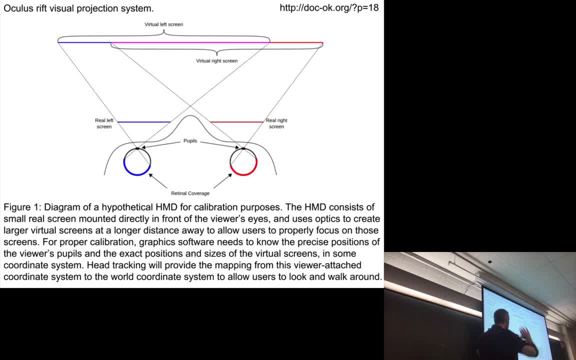 So we've got two very small real screens mounted directly in front of the viewer's eyes and we need to use optics to create larger virtual screens at a further distance away. What do they mean by that? When your eyes see light, manipulate that to change the way you see. 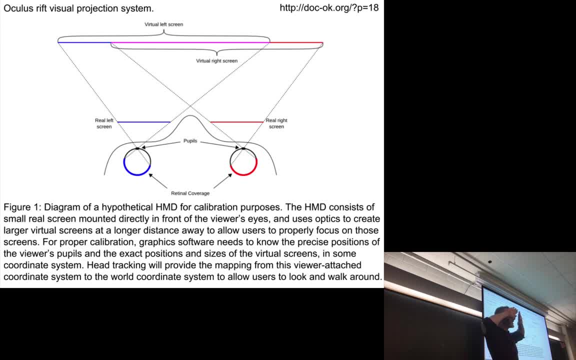 Right. So when this is working, when you put on the goggles, you do not see two screens directly in front of your eyes. You see some other scene which is further away from you. How do they create that illusion? How does it look to the wearer that the scene is actually further away than it actually? 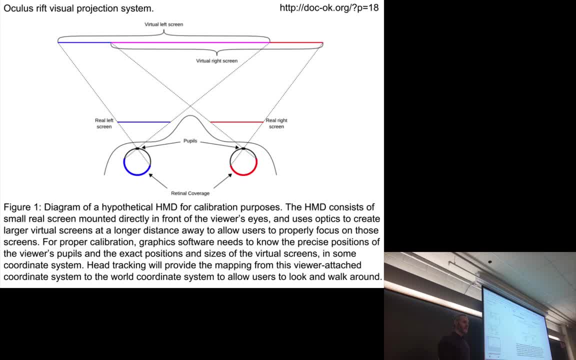 is They use lenses to manipulate focal length. They use lenses for the focal length. Yeah, that's important. What else If you were creating the graphics that are going to be painted onto this blue screen? the left blue screen and the right? sorry, the left real screen and the right real screen. 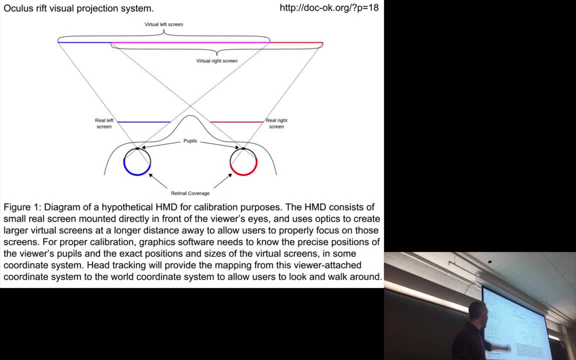 what graphics are you going to draw to help pass the illusion that they're actually looking at something that is further away? So if I was going to wear goggles at the front of the room here, you could take the view from my point of view, cut it in half and paint this half of the room on the left screen. 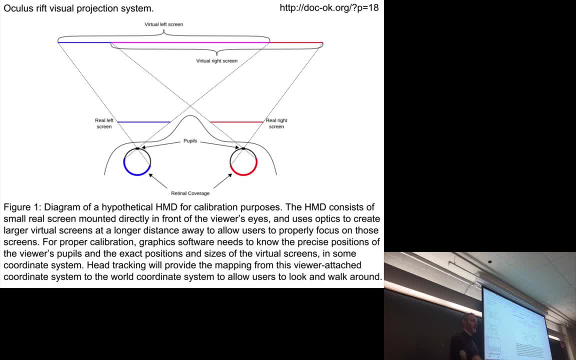 and the right side of the room on the right screen. Will that work? You can probably tell by the way I'm posing this question that it won't. Why not? Absolutely not. It's not going to work. It's not going to work. 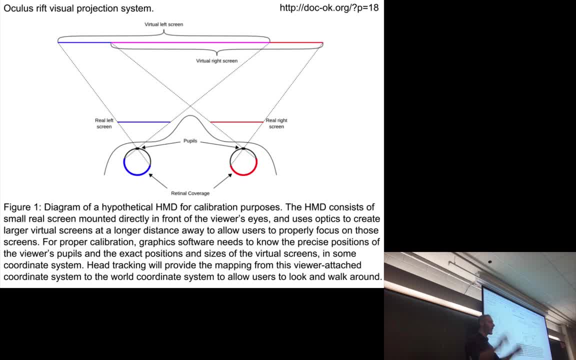 Absolutely. There's some overlap right, So I am looking at all of you with both my eyes and there is significant overlap. What can you tell me about that overlap, The differing lengths and the differing amounts of objects, and how far away it is? 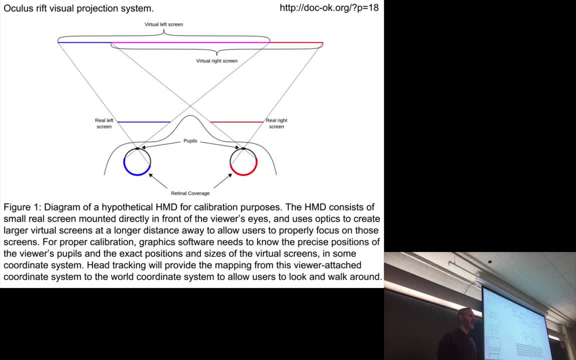 Absolutely So. when I'm looking at any one of you, I'm actually seeing very slightly different views of your head, Of your head with both eyes right, So it's not just overlap, it is also slightly different views And, if you get that just right, if someone is looking at an actual 2D screen or a pair, 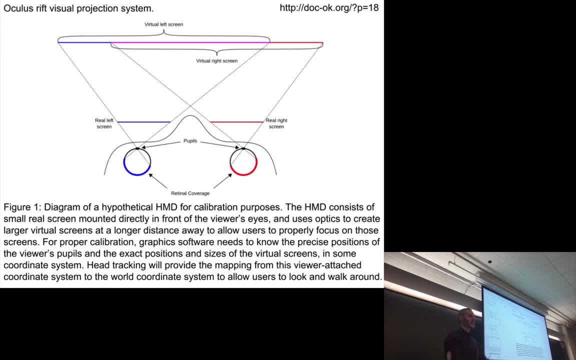 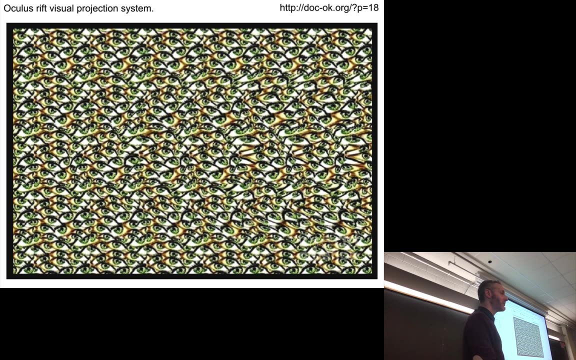 of screens very close, it will cast the illusion that they're looking at something further away. It is actually. if you put the right pieces in place, it's not as hard as you think. What is inside this picture? Just a bunch of eyeballs. 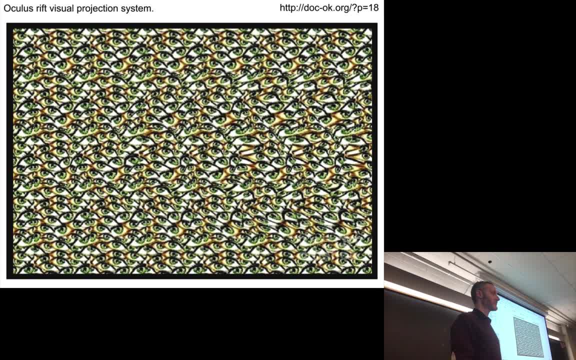 Just a bunch of eyeballs? Not quite So for those of you that have done this puzzle before, there is a trick to see the hidden object. What is the trick? You kind of like put your face closer to the picture and then move it a little bit. 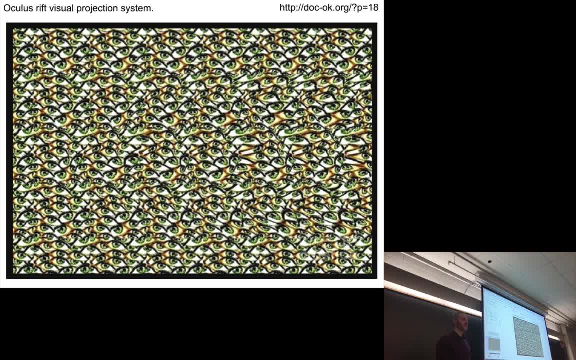 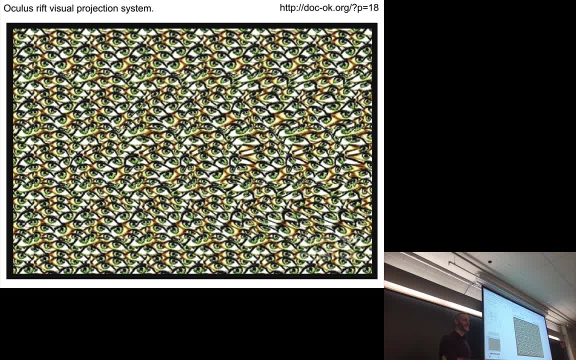 There's an easier way to do it, where you don't have to leave your seat: Relax your eyes. Relax your eyes. When you relax your eyes- and again we want to be very specific about the visual system- when you relax your eyes, what happens? 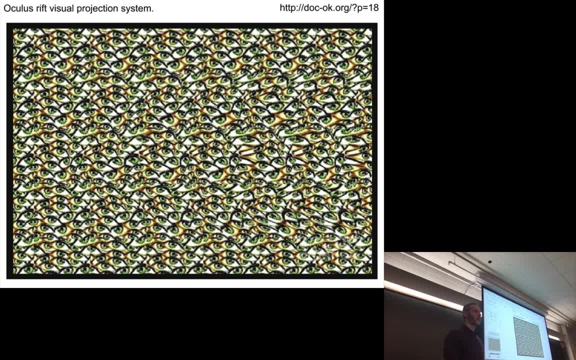 You're changing your focal point. You're changing your focal point Exactly Right. So your pupils? I'll leave that up for you to give it a try. Relax your eyes. Don't look at the screen, Look through the screen. 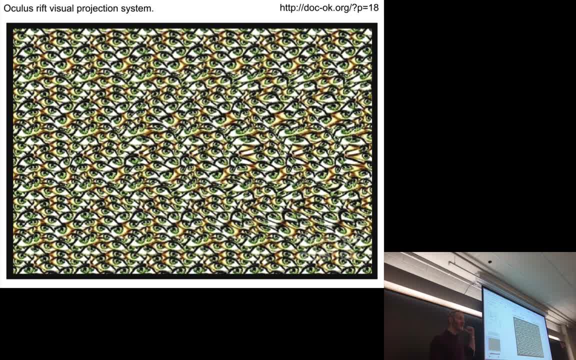 I don't know how it looks from your point of view. You might have to look a couple of feet beyond the screen. When you relax your eyes, you'll no longer be looking at the screen, but you'll be focusing on a point behind the screen. 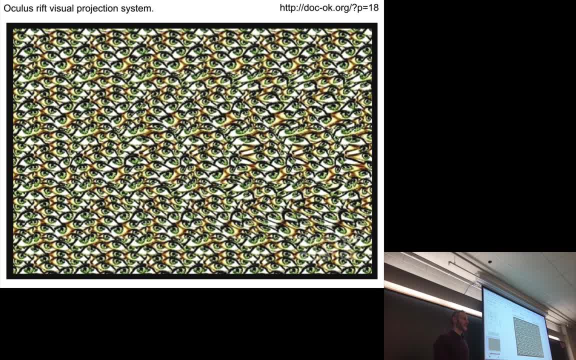 And when you do, you will see Anyone manage to do it. yet No, It may be because it's on the screen far from you. Maybe you do need to be closer. Okay, Well, you can try it at your leisure on your laptop with the screen a little bit closer. 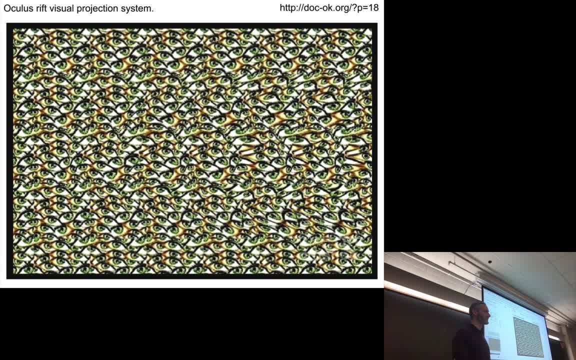 I won't tell you, I won't give away the surprise. No one can see it yet. What's that? A clue as to what's inside. It's another giant eye. Not that exciting, but there you go, Okay, Okay. 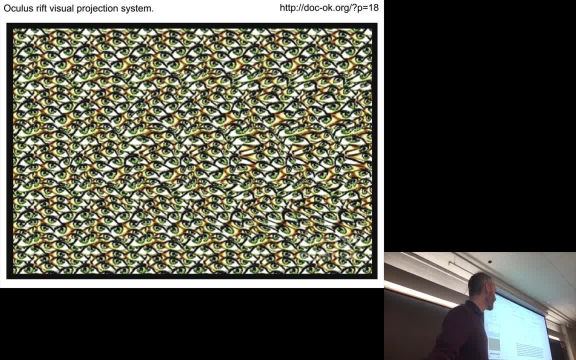 No, Okay, All right, You can play these at your leisure. There's a gazillion of them on the web. One of the tricky things with goggles is you need to detect not only head position and orientation and acceleration. you need to be able to detect the position of the pupils in the user's eyes. 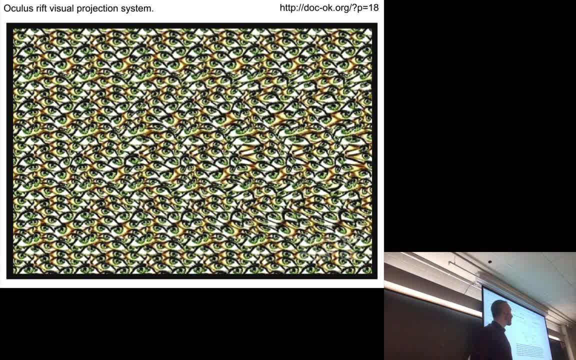 Where are they looking and how far away are they looking? So in this top-down display you can see if the pupils are more or less parallel. If you took lines emanating from those pupils, they would cross at a very far distance away from the eyes. 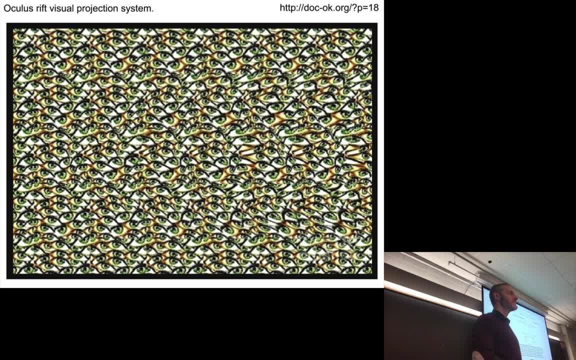 They're looking at something far into the screen and you would have to adapt what the images you're painting on the real screens to bring into focus that distant object that they're looking at- Not this one, Not back to this one. 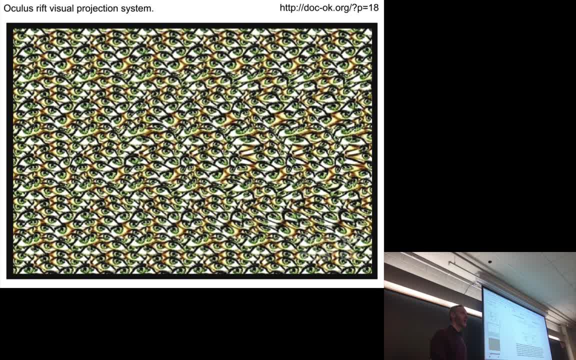 Someone is wearing these VR goggles. Where are they looking? What are they looking at? They're looking at the little images, but from their point of view, they are looking at a larger scene, the one that's behind these two screens. Actually, this might help. 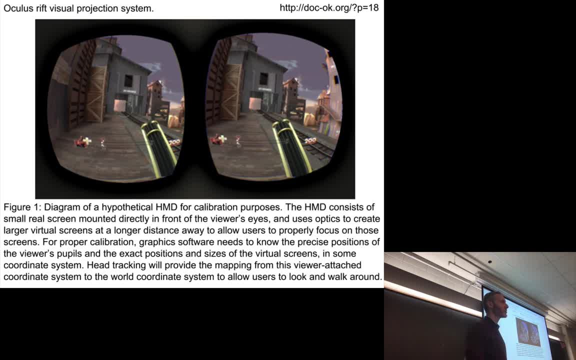 Here's just a screenshot of what you see from virtual glasses, And you won't be able to do it because you're not wearing them. But if you look carefully, obviously there is a fair bit of overlap between these two images. These are the two images that are drawn onto the real screens. 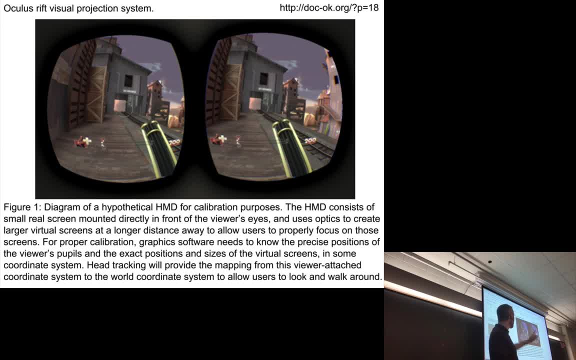 If you're wearing these, they overlap and it looks like you're looking at this actual scene. but you see it in 3D, You'll notice. not only is there just simple overlap, but the objects are rotated slightly relative to one another. 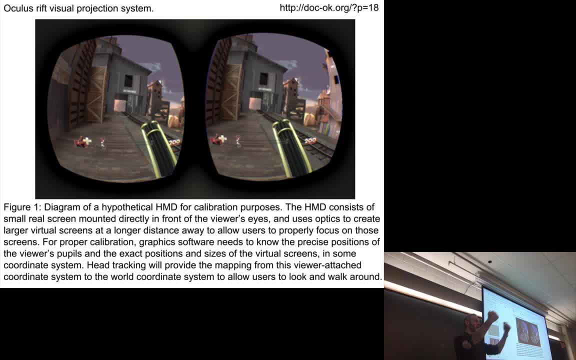 Because, again, when I'm looking at one of you or when you're looking at me, your two eyes are seeing slightly different angles of my head. Same thing with the objects in this scene. So you're seeing this, but the user who's wearing these goggles is seeing a scene that's much further away in 3D. 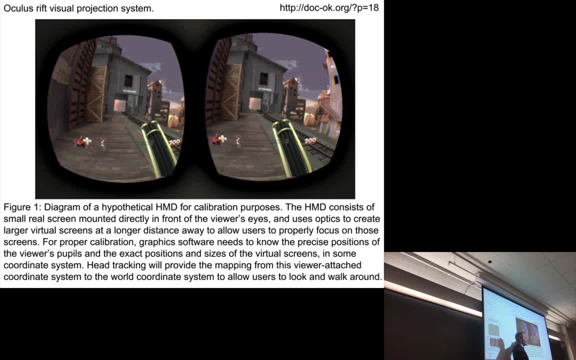 The user who's wearing these goggles is seeing a scene that's much further away in 3D. The user who's wearing these goggles is seeing a scene that's much further away in 3D. The user shifts their saccade. 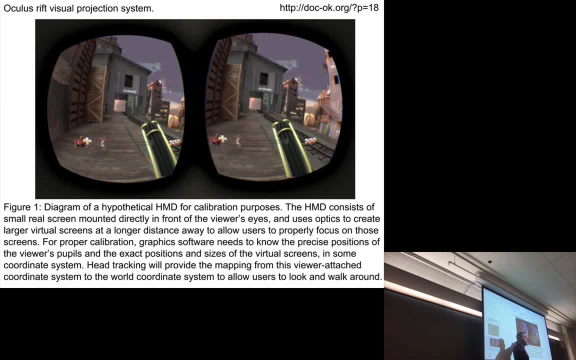 They are looking at this object, which is close, and then their pupils change And it turns out that they're actually looking at that object in the back. You might need to bring one or two into focus or maybe move the whole scene. 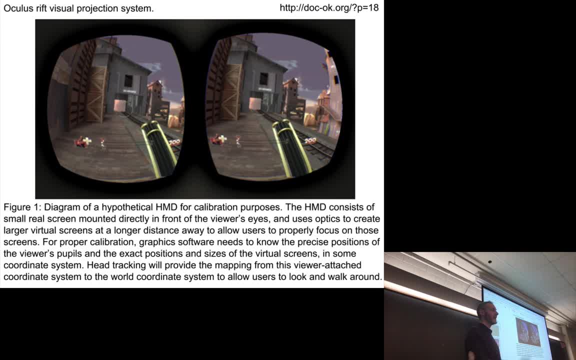 If they move their head and rotate their head, we need to rotate the scene. Other objects need to rotate at different speeds. It gets tricky. I'm just curious: Have you figured out the exact angles of your eyes or what the difference is? 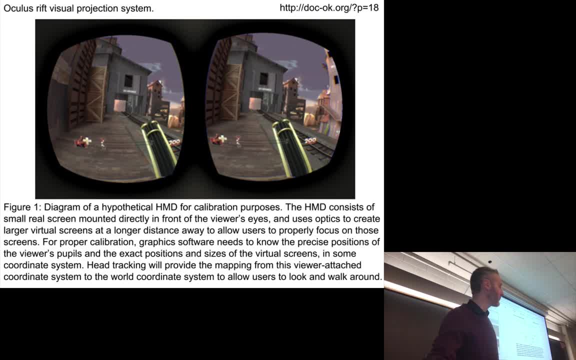 Sure, Different goggles have different solutions, but it's an easy one. You have a small camera sitting on the inside surface of the goggles looking back at the user's eyes. It's a pretty easy computer vision problem because you have a field of white. 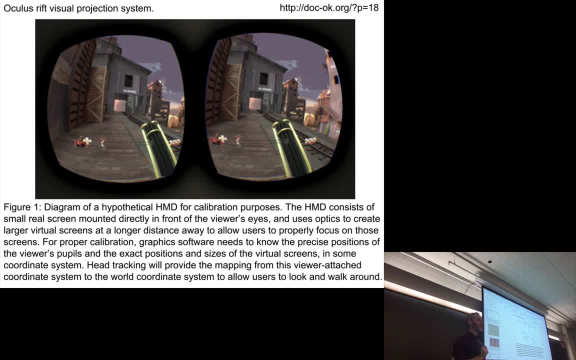 with something dark in the middle. You remember, when we talked about social robots and we talked about joint attention, There was a robot that was actually looking at humans' eyes and was trying to detect what object the human was looking at. Same thing here. 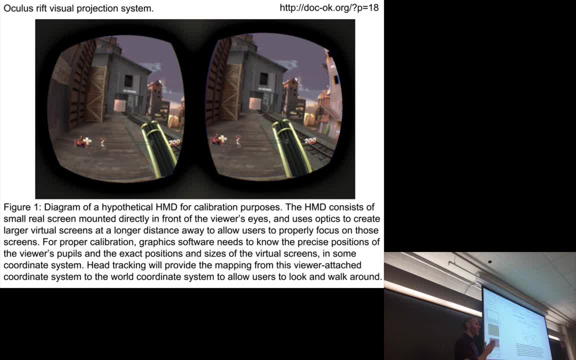 Not too difficult. You might also remember we looked at a video by Johnny Lee where he had a Nintendo Wii remote that he was wearing on his head and as he moved his head, the scene on the screen moved in opposition. If you're looking through an empty window. 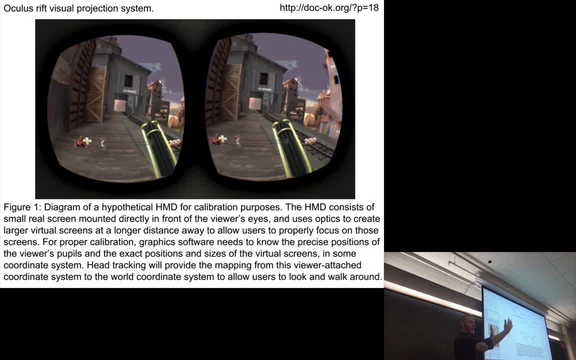 and you move your head, the scene that you see through that empty window, through the frame of that window, changes. You can play all those same tricks with the Google glasses. Does it break if you go cross-eyed or something? Good question, I don't know, I haven't tried it. 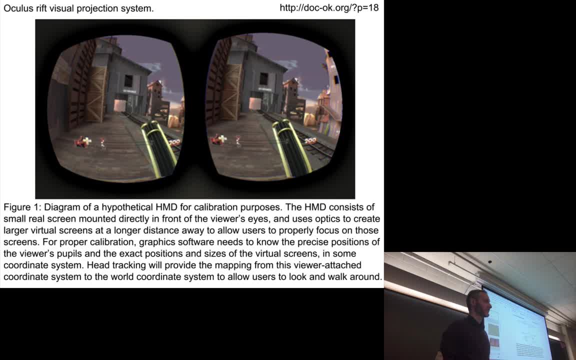 Probably yes. So then someone who has a lazy eye or something might not be able to use. How do we support people whose visual system deviates from the normal functioning of a human visual system? Absolutely Okay, I think, in the interest of time. 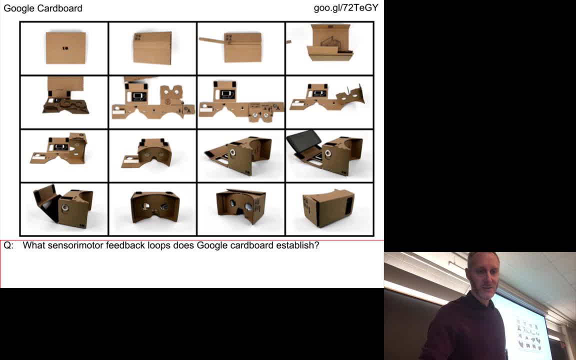 we'll skip over. Let's see How much more do we have here? Yes, In the interest of time, we will skip over Google Cardboard. This is a great one, because as long as you have a smartphone and some cardboard, 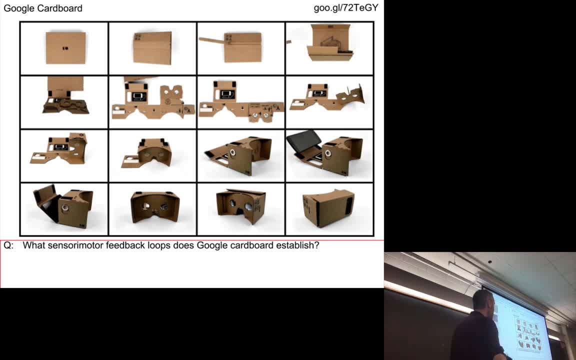 you can try this out yourself. It's not sophisticated, but it's got some of the basics that we've already talked about with stereoscopic vision. Pretty neat idea there: Google Cardboard. If you do try it out, play the same game we did. 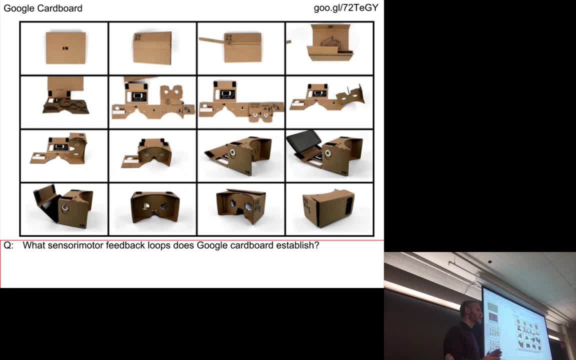 with the five VR systems? what aspects of visual repercussion in response to head motion is supported or frustrated by Google Cardboard? Has anyone tried it out before A couple of people? How was the illusion Not bad? So-so Better than you thought. 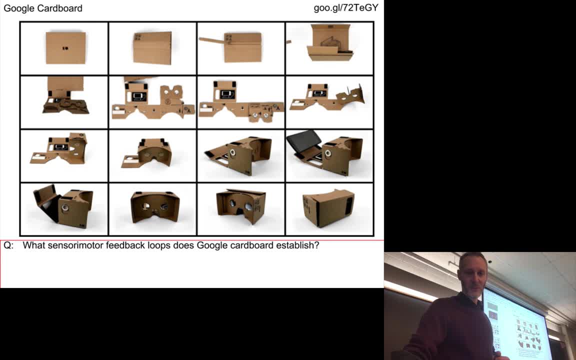 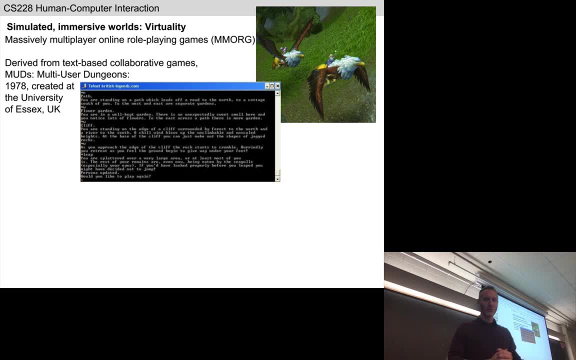 Better than you thought. Okay, there you go. Okay, so we talked a little bit about the cutting edge of VR. Let's go back in time to virtual worlds. The very first virtual world was a multi-user dungeon, or MUD. 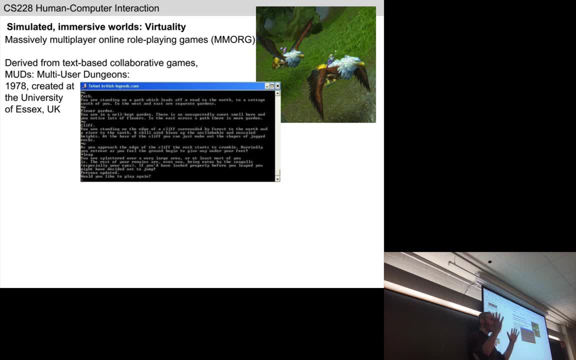 created in the late 70s in the UK and it was alt text. Again, we've had books for a long time, so virtual worlds were actually. if you go back and look at the history of video games, were pretty smooth. 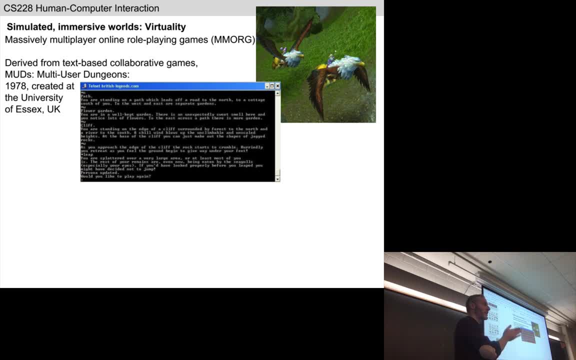 pretty smooth progression from a story in text to what we have today. right, The graphics are nice, but not necessary. not necessary, Okay. so let's look at a few virtual worlds now and think about what might be the killer app. So we've been promised VR. 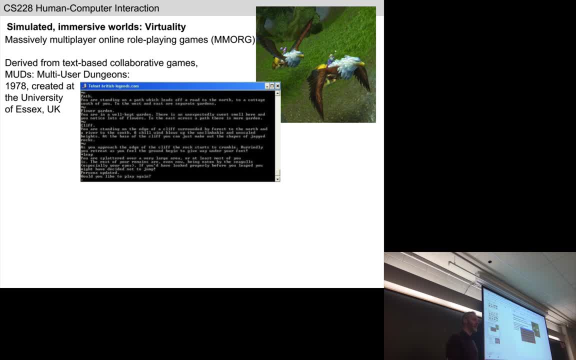 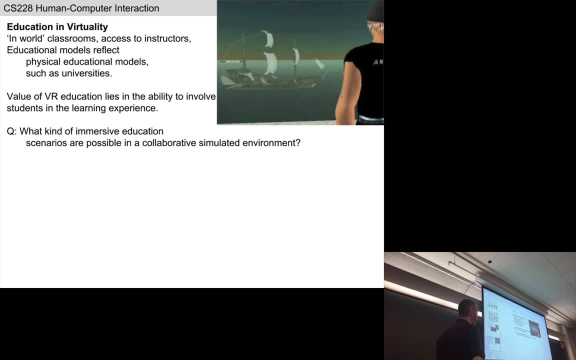 for a long time. We now have pretty sophisticated computer games. What can we do with them other than play a game? Those in academia have thought for a long time about how we might use VR to improve the learning experience. I'll show a bit of this video. 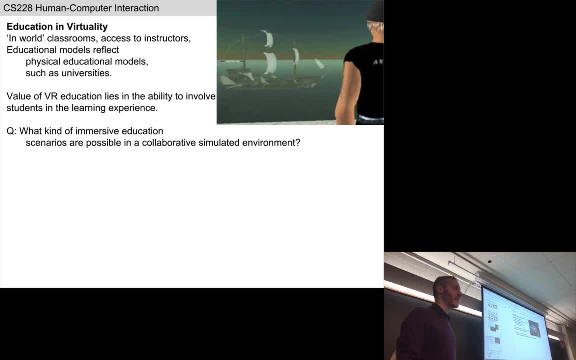 This is a promotional ad from Ohio University that built a virtual version of their university in Second Life, and I will switch back to my other machine because this has some sound- Not great sound, but some sound. It would have been nice to fly to campus this morning. 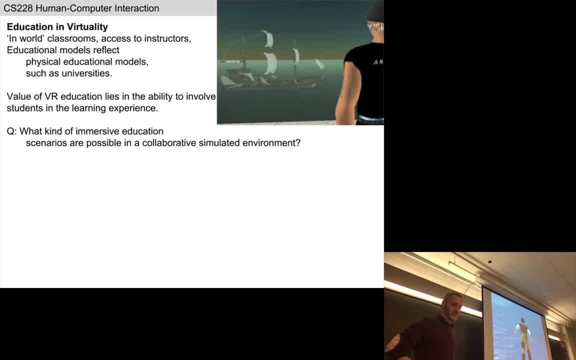 Most of us have dreamt of flying. We've dreamt of a world with endless possibilities, where reality falls away to be replaced by imagination, creativity and endless opportunities for discovery. Discovery, so central to learning, has now broken free of the boundaries of the classroom. 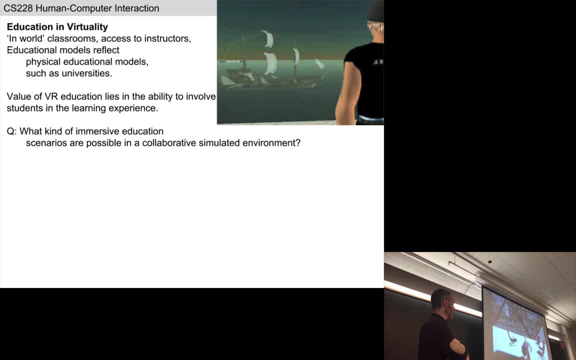 Learners now thrive in an environment unbridled by space, time or even the laws of physics. Welcome to the Ohio University Second Life campus: an engaging new universe of learning, opportunities for intellectual and professional growth, an immersive atmosphere where the classroom has not just been recreated. 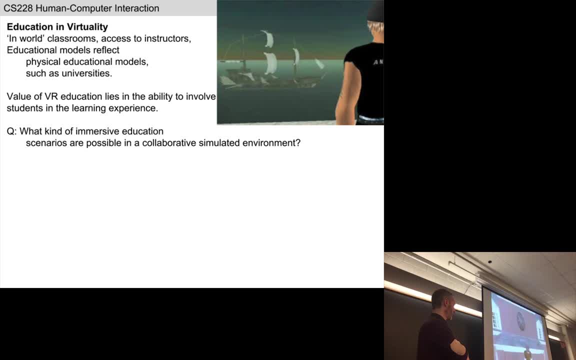 but rather reinvented. Learning experiences can range from entire college courses to one-hour learning modules. Learning comes in many forms. Learning kiosks are scalable systems for housing course content, for blended or stand-alone delivery. Each course and each kiosk houses applicable course content. 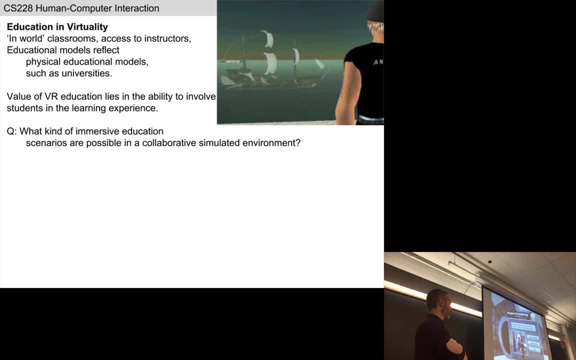 in a variety of possible media forms, from text to video, podcast and more. The campus also contains substantial space for virtual trade shows and conferences. Second Life conference exhibits are a highly cost-effective method for ongoing contact with your customers. Art and music is alive. 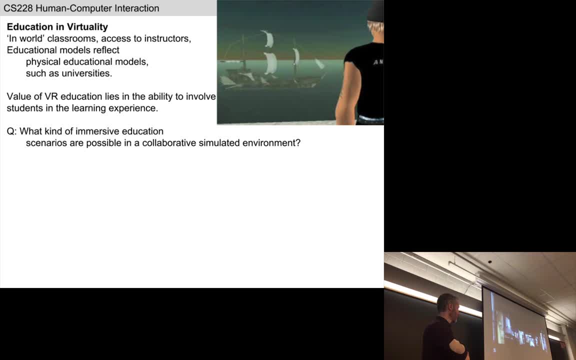 in the Arts and Music Center where artists, filmmakers and musicians from Ohio University and all over the world display their talents. The Campus Student Center is where real-world student activities are enhanced by the rich collaboration made possible by Second Life At the heart of Ohio University. 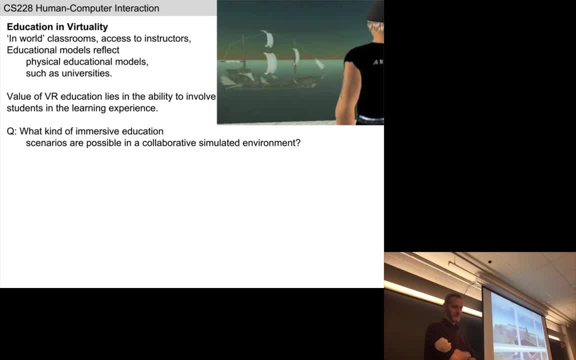 and Second Life is the same mission that drives Ohio University in real life: a complete dedication to the learning outcomes of our students and industry partners. Don't just dream of flying, Spread your wings and explore the Ohio University Second Life Campus, where discovery is limited. 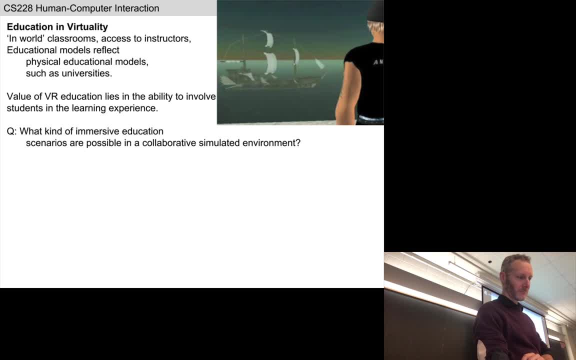 only by your own imagination. Okay, discovery is limited only by your imagination. You can have rich interactive experiences in the virtual Ohio University, like facing each other and typing on virtual keyboards. I think conceptually it's there, but like you should make you act it. 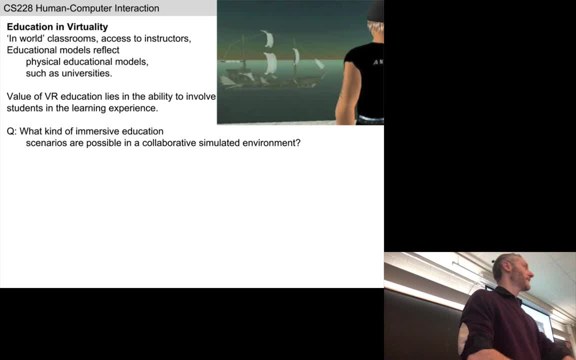 How so? So I think, like the idea of a virtual education and being able to like have like that experience would be great, but like I feel like in 2018, those graphics are, like relatively unacceptable and like you know what I mean. Alright, so we take that system. 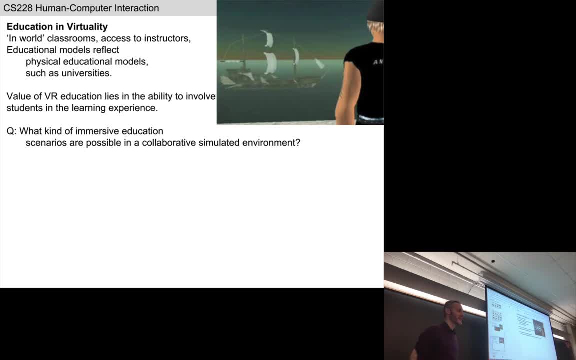 and we update the graphics to 2018 levels and we expose the students in the virtual campus to a campus building where you go inside and there's an internet kiosk with a virtual screen inside and virtual buttons and some professor sitting in his office lecturing at you. 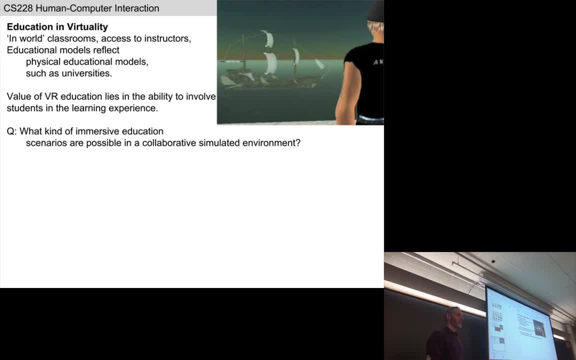 Again, this one's a little bit dated. we could update that, Not to pick on Ohio University. but again we have this brand new technology and it's difficult to think about the physical and cultural context of learning Right. So we could, for example, create the same old standard. 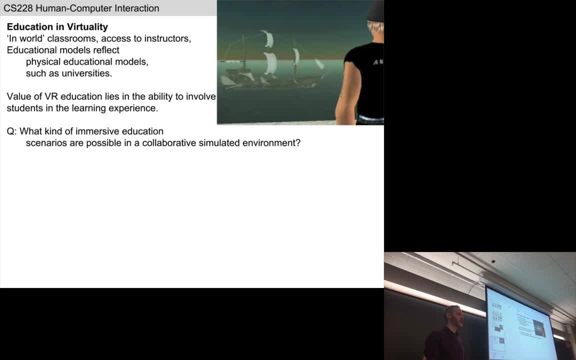 approaches to education in a virtual system. but we're kind of missing the whole point here. What aspects of physical, cultural and social interaction are missing from this particular virtual world? that would facilitate learning What's missing from what's happening right now. that would help. 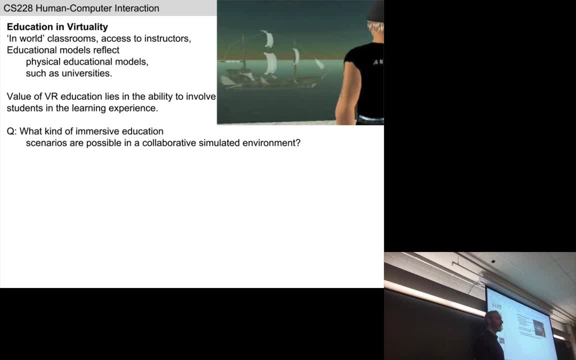 your learning. Eye contact, Eye contact. I can't maintain eye contact with all of you in parallel, Right, So the professor avatar could meet with the student avatar and, assuming they had facial expressions, maybe it would be easier for me to maintain or have one on one. 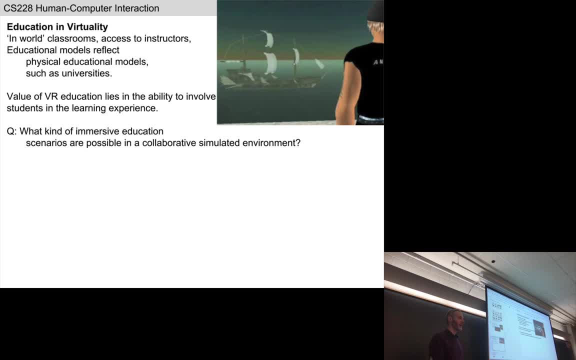 interactions with you more often, rather than you making the five minute walk out to Ferrell for one hour a week, possibly. What else? You have a way to like a student's VR and theoretically have a virtual three dimensional model, Which they do have in Second Life. 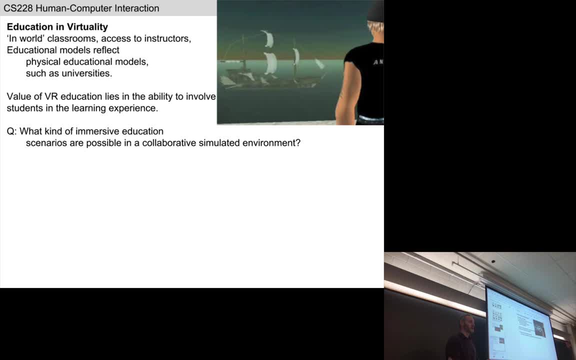 right, Or World of Warcraft, wherever we're going to host our classroom right, It is a virtual 3D world. It may not feel like it unless you're wearing goggles, but if we do have a three dimensional environment, what could we do other than? 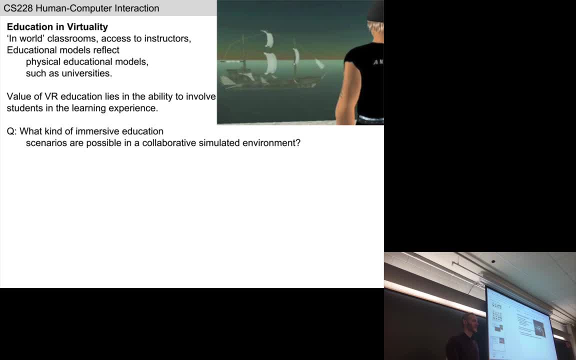 create another virtual lecture hall and have all the student avatars sit in virtual desks and listen to the virtual professor. This is kind of tangent a little bit to what you said recently in the news that there was a professor of history that was teaching through the 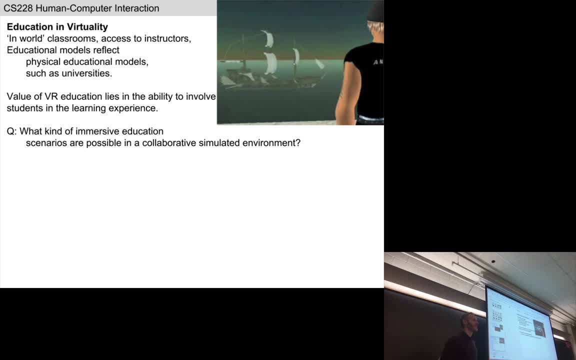 architectural architecture by showing them like that in video games: Show rather than tell. Yeah, Absolutely Right. So if we're dealing with physical artifacts, architecture or art, it would be great to be able to show rather than tell. That's one of the 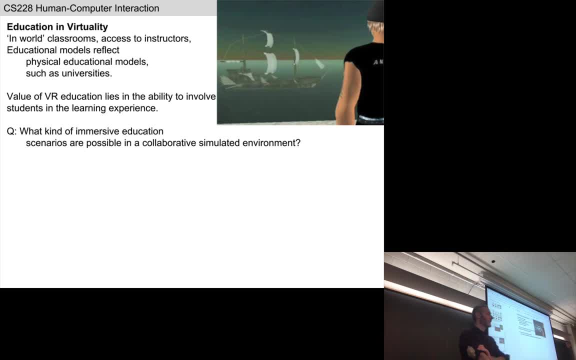 possibilities that virtual reality may afford in an educational setting. You would need some like pretty impressive like chat box to be used, Assuming that there isn't someone on the other side of the avatar. you mean, Yeah, Right, Okay, So we could try. 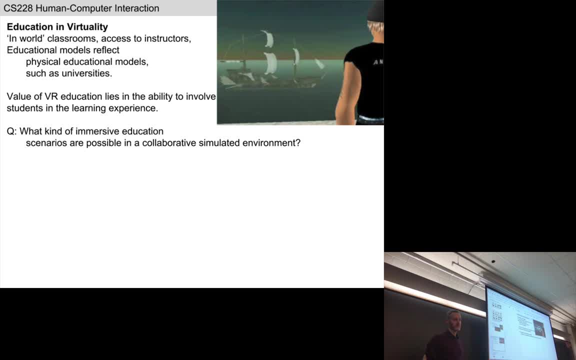 and automate things again. Right, And maybe we would need a sophisticated chat box Like this seems like a good idea versus like physical disabilities, because things like this would be hard to get around campus, Possibly. So if you can't make it to campus, 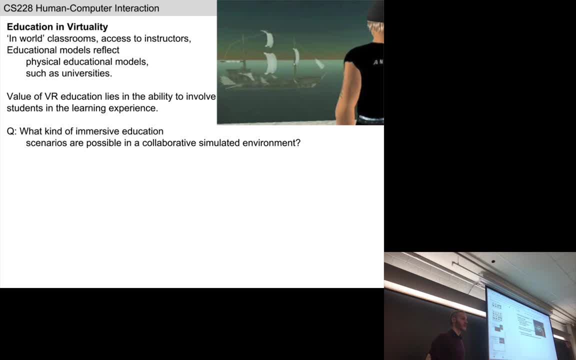 reaching students that have limited mobility. absolutely What else? What are some of the things that may be possible with this kind of technology? It could be really good for like foreign languages to you know, like mic chat, you know you can talk to like native speakers. 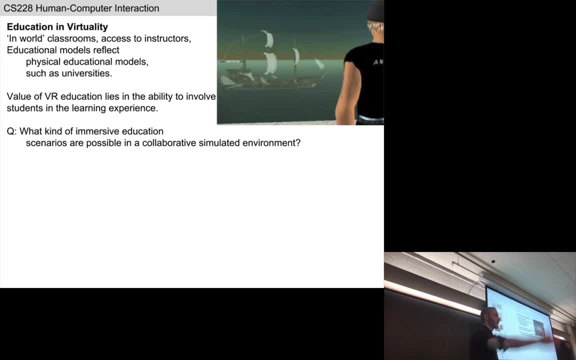 you know, you can have native Spanish speakers teaching a class with American Spanish. Absolutely, Yeah, There's an idea: Absolutely For training, for training purposes, Right. So show is better than tell and do the actual sensory repercussions you would get if you were performing. 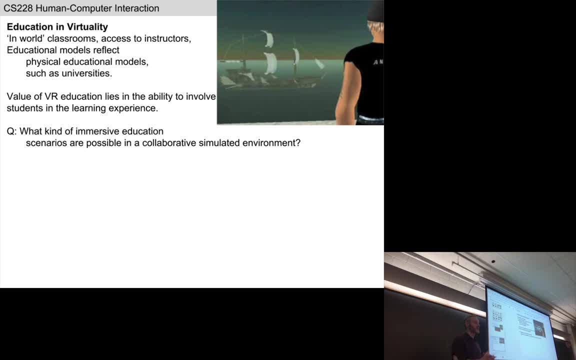 the actual surgery. So virtual reality is making inroads in terms of training very high skilled, fine motor tasks like surgery, learning an instrument and anything like that. Okay, So that's education. Again, we're all here physically, so VR hasn't made it to education. 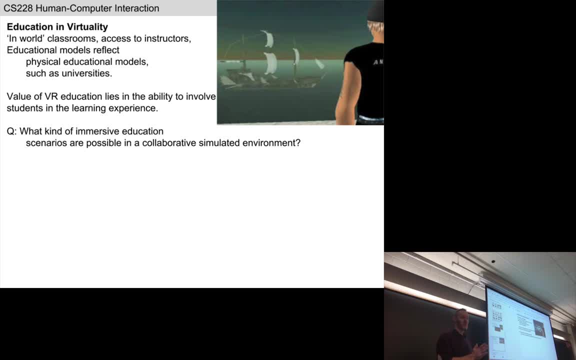 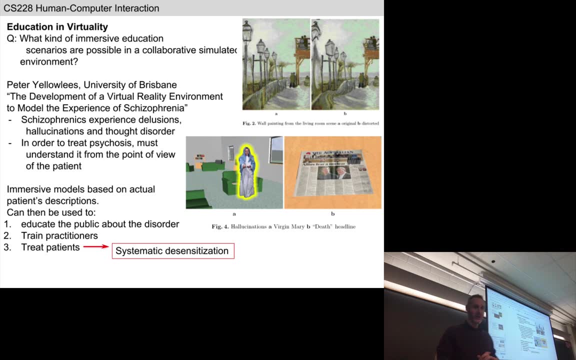 on a large scale yet, but it may be possible. We just talked about medical training. There is a lot of use of this in terms of education for medical pathologies. There's a great example here. This is a snippet from a research paper a few years. 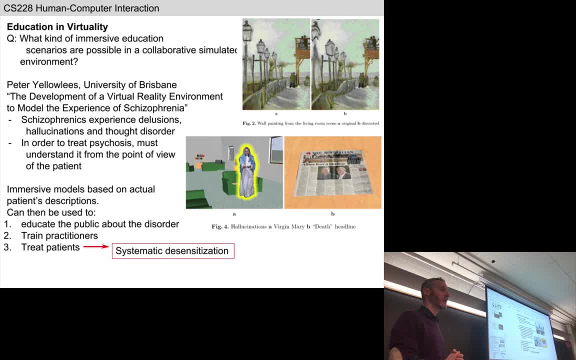 back about using virtual reality to train students about schizophrenia For a lot of mental disorders. if you're learning to try and treat someone that suffers from a particular mental disorder and you have that disorder, it is very hard to relate and provide care. So could you create? 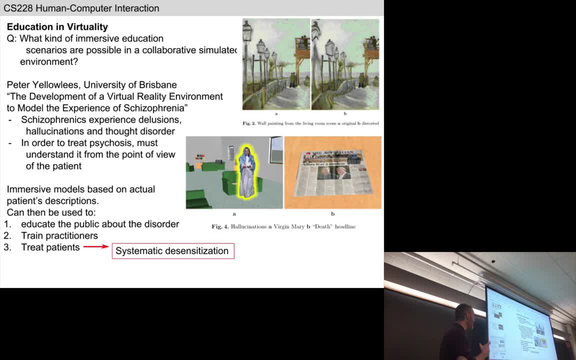 a virtual environment. it may not be a very pleasant one, but it may be as close as possible to what someone who suffers from schizophrenia or delusional disorders might actually experience, and you can then put students in the shoes of what it feels like to suffer from that. 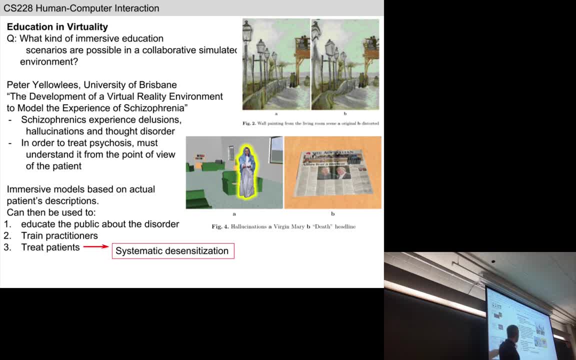 disorder. So this is a wonderful educational experience. We could help to educate the public. so, assuming that this system is relatively accessible, we could build up empathy for particular disorders by making it easier for people to put themselves in the shoes of the person that suffers from that. 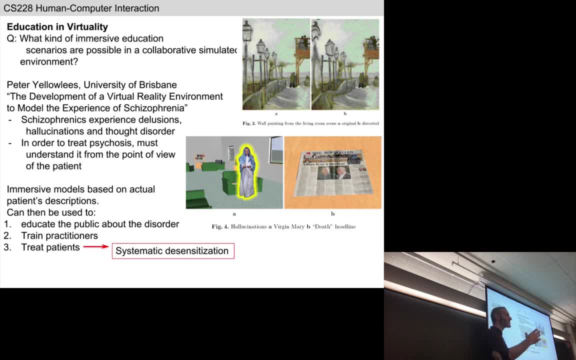 pathology. Again, we could use it to train practitioners to think: what are they feeling, what can you do in that moment to help. and then also you can use it to treat the patients themselves. If you suffer from schizophrenia, for example, you can be fitted with a system. 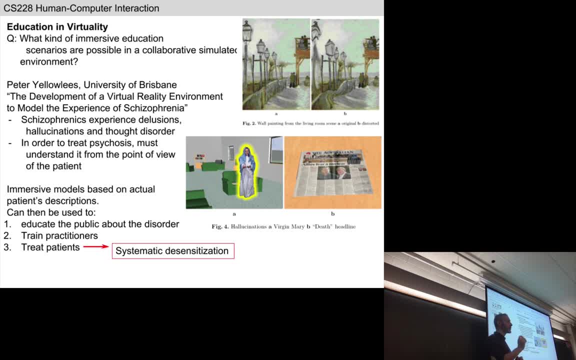 again in the presence of experts, where you can very gradually turn up the realism, You can implement or turn on an episode and you can try, if you do this in a systematic way, to desensitize the observer, to the effect One of the things that's. 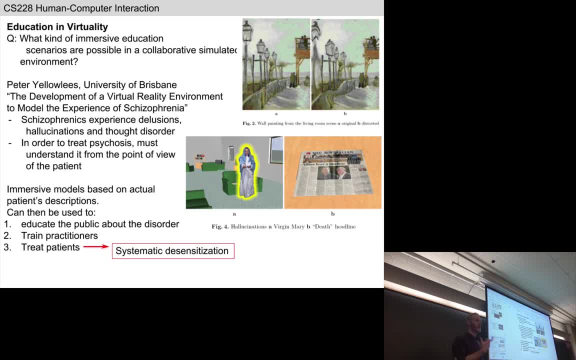 most debilitating about mental disorders is lack of control. You have no control over when an episode occurs. Imagine you are instrumented with technology where now you have control. You are holding control over the magnitude of realism of that event. You might be able to gradually 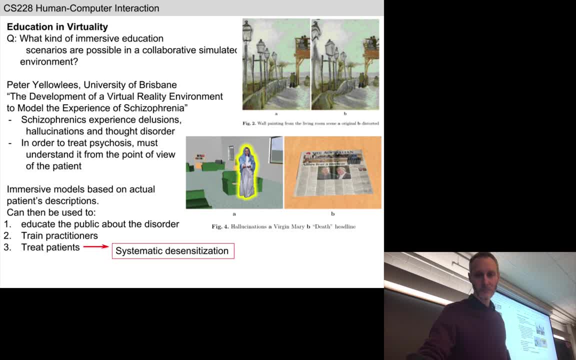 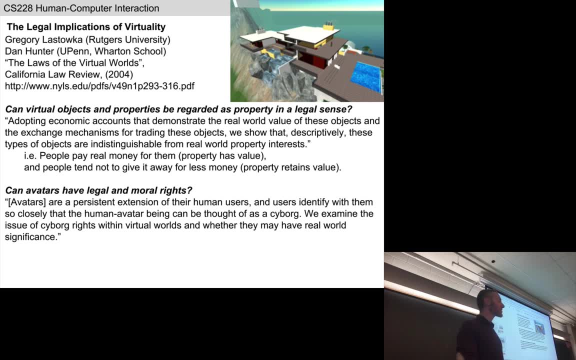 desensitize yourself to that event. Okay, What else is possible in virtual worlds? Well, the law is getting involved. There's some interesting papers from legal scholars about virtual worlds. This is again an example of what we can do, For example: 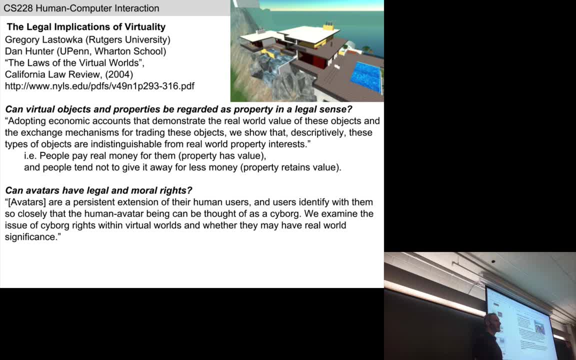 in a virtual world. if you have virtual objects or virtual properties, are they property in the actual legal sense? If you build a beautiful oceanside home in World of Warcraft or Second Life and I come along and knock on your door, I guess it?